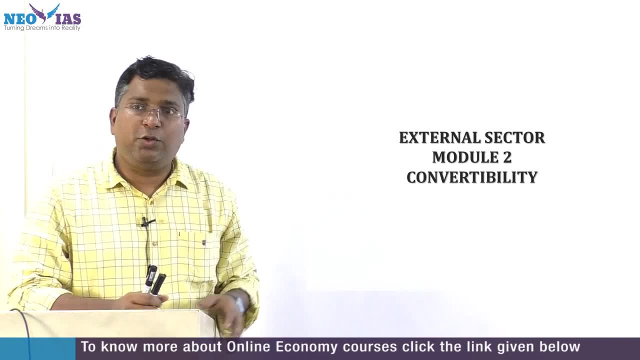 this also, there have been 7 questions been asked in 2020.. So, from in 2020, module 1, there have been a question. From module 2, there is a question. Module 3, there is a. 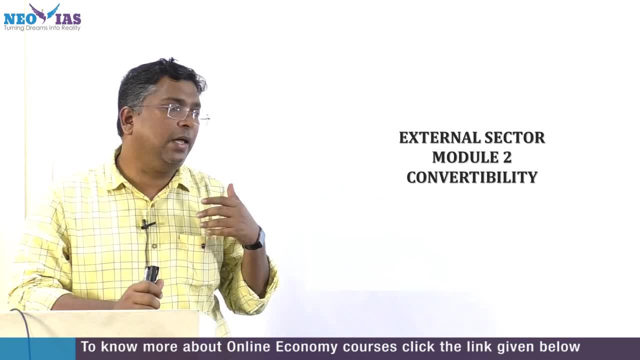 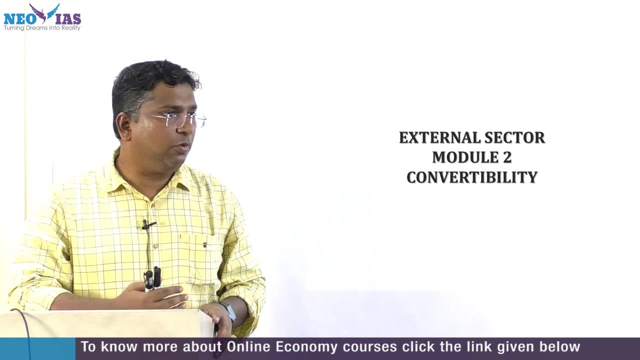 question. So last year external sector have been very important. ok, All were conceptual questions, Even though questions arise because of current affair. all were conceptual, Even if you have not read the current affair. but you have if you have gone through our class. 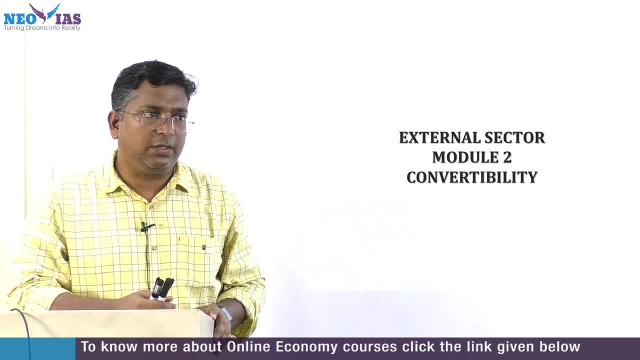 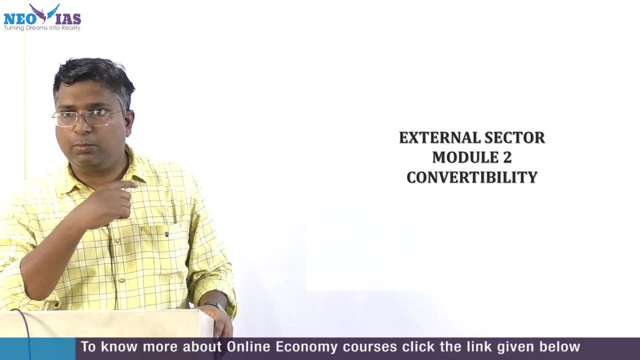 notes and material and classes. that will be sufficient. ok, But to understand this module, anyone who have not attended the module 1 classes, they will have a little bit of problem. All were there. no Balance of payment. you were there. You were there. 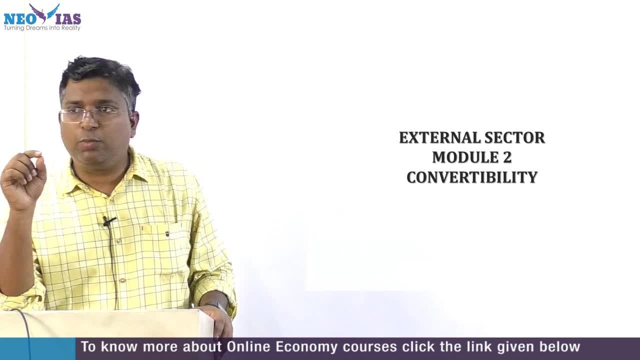 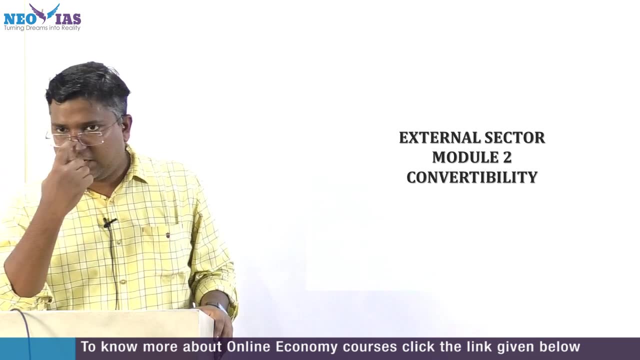 Ok, So what is what we studied in module 1 under balance of payment? what I told you? it is an external account. All the external transactions of the country will be reflected in that account in the form of receipts and payment. All the exports are receipts, All. 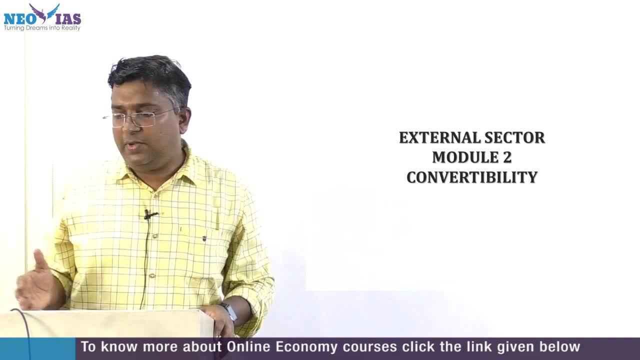 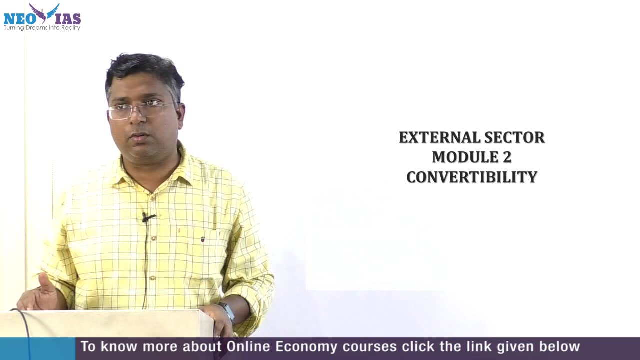 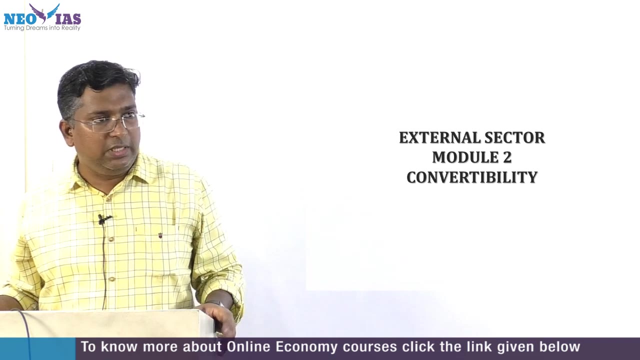 the imports are payments. ok, Then it we have. we have studied the components of current account and components of capital account. There have been question from the components of current account as well as capital account. ok, Now what about here? the the, the base amount, As per the previous part, which is 2,, 5,, 4,. 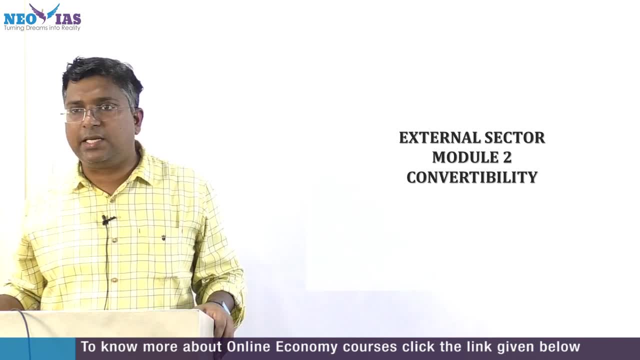 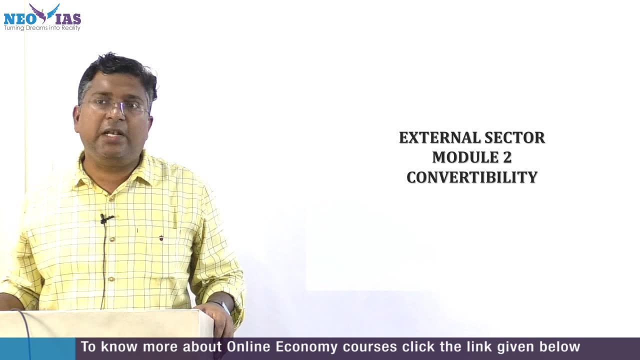 5,, 6,, 7,, 8,, 9,. okay, This is the base amount which we have collected. So when, how much has been collected from the previous part? It is a total amount- And from the previous. 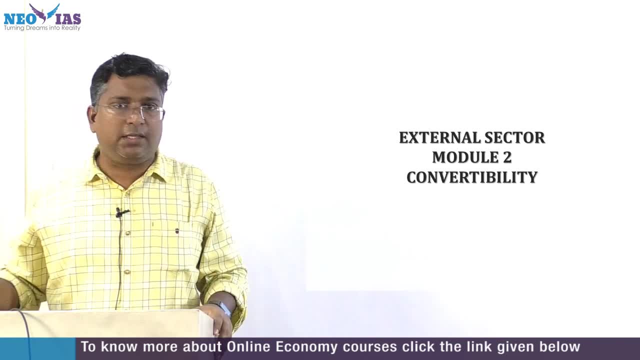 part you have taken. you have taken crossfreight. right, It is not inside the previous part, the previous part, Ok, Ok, You have taken the crossfreight. Ok, Ok, Ok, Ok, Ok, Ok. 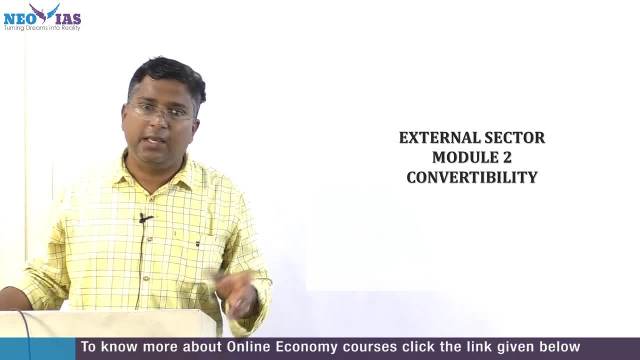 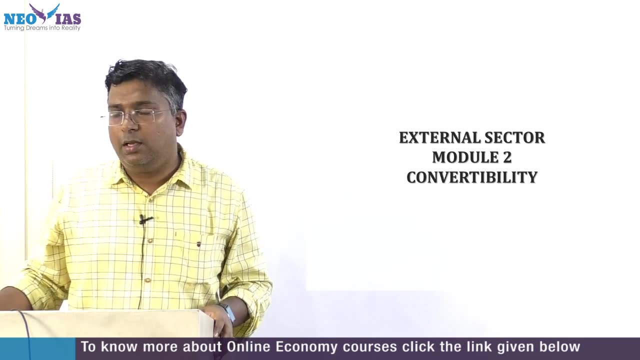 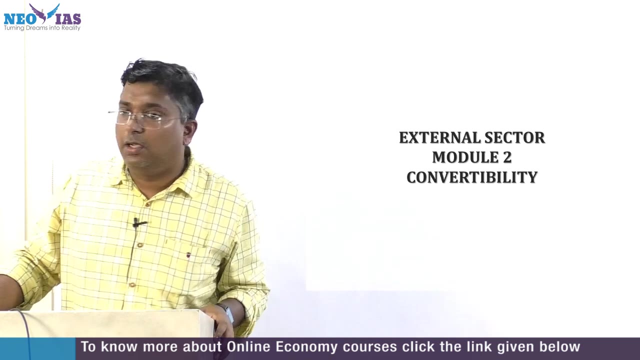 Ok, Indian rupee. like Pakistan, there is Pakistan rupees there in Nepal, Nepal rupees there. okay, but in India that legal currency is Indian rupee. now, but when? if we do external transaction? if we do external transaction, what will happen? Indian rupee will not be accepted. Indian rupee. 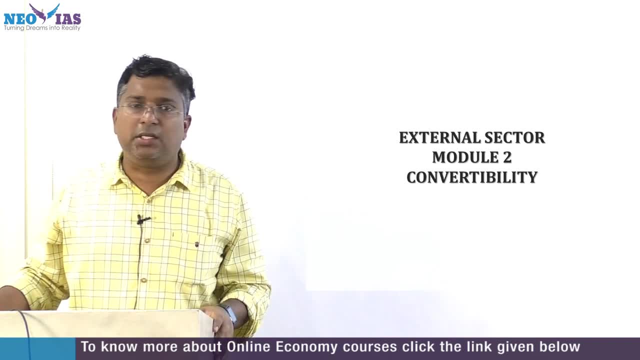 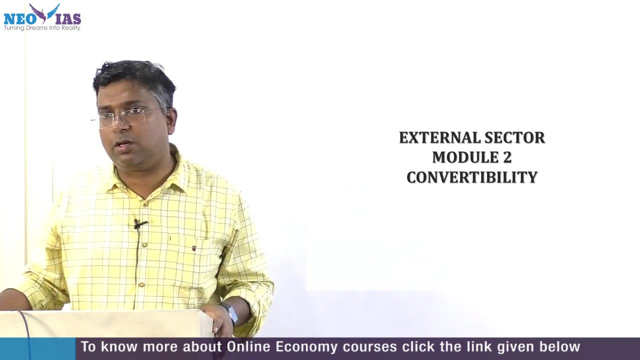 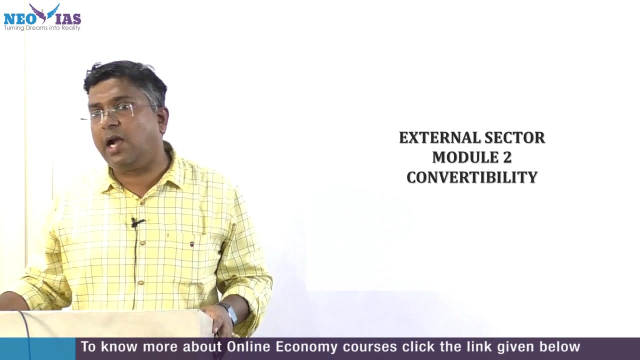 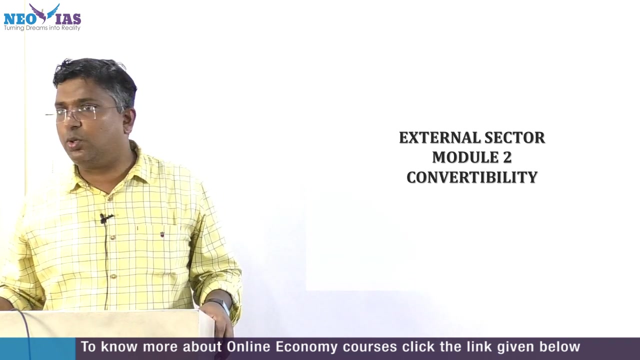 will not be accepted. it should be for all the external transaction, that is, all the export and import transaction which is mentioned in the current account, as well as all the receipts and payment in the capital account. it should be through a commonly accepted currency, what we call it as hard currency. okay, so when we do external trade, that is, export and import both- 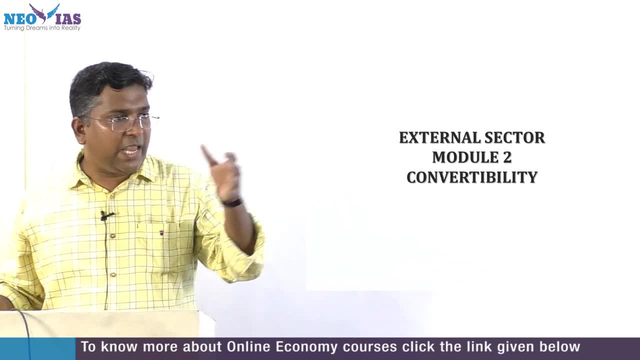 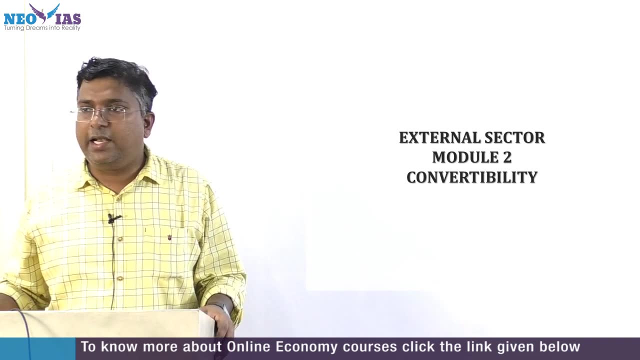 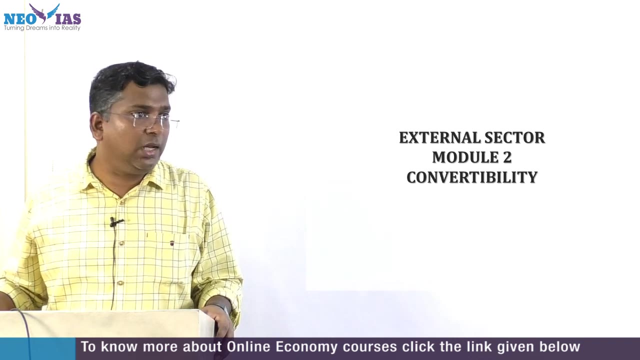 in goods and services, as well as when there is capital movements between two countries or more than two countries. everything will be reflected in the balance of payment. okay, and I told you, the most prominent global currency not we use as well as other country uses US dollar, so US. 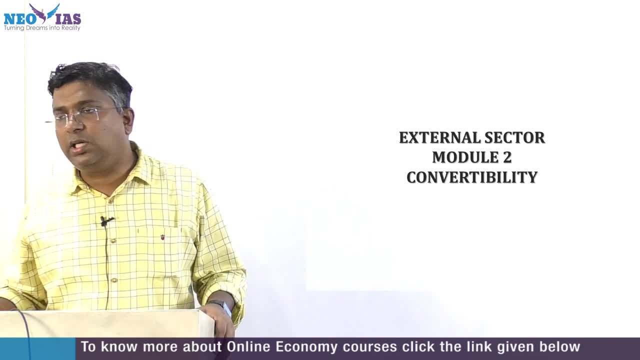 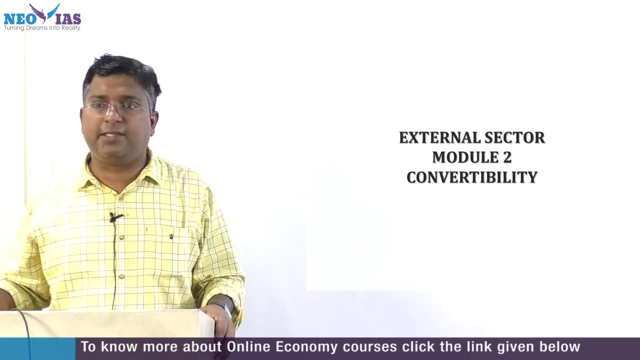 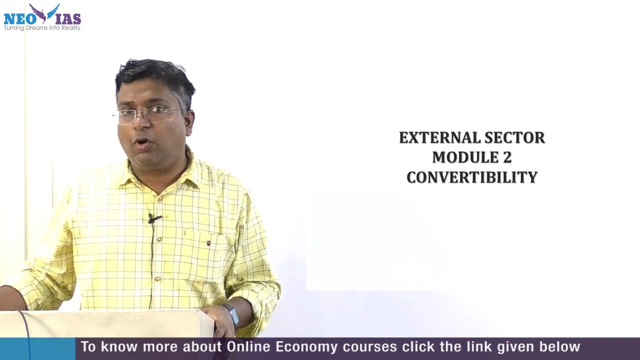 dollar is a hard currency. okay, so almost all the in India, all the external transaction is reflected in dollars only. but it doesn't mean that only with dollar only we transact. we transact in euro, we transact in Japanese yen, we transact in pound sterling, etc. but what we will do, we will. 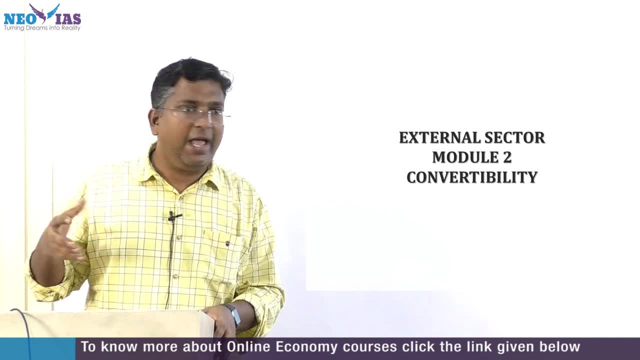 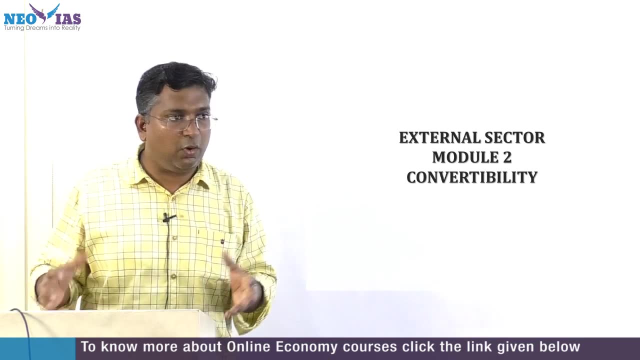 convert all those currencies into dollar and we will convert all those currencies into dollar and we will say that this much so. currently we are having a total foreign currency assets. this is a word we use. foreign currency assets is one of the major component of Forex Reserve. its denominated 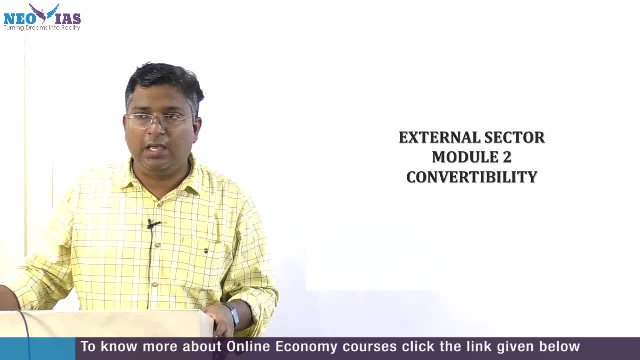 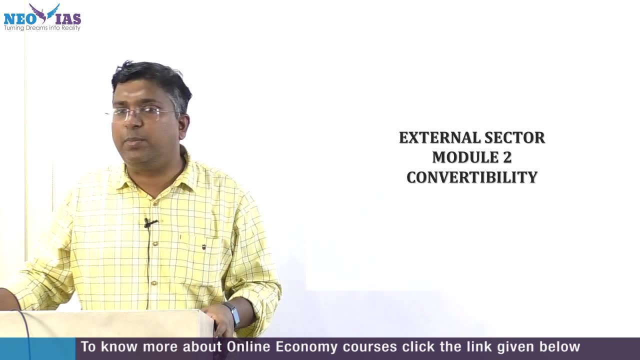 in dollar. BOP is denominated in dollar. okay, so why these? why US currency or European currency was selected? is that their value is almost stable. as features of an hard currency is that they are not volatile. Their values almost stable. Their values almost stable. 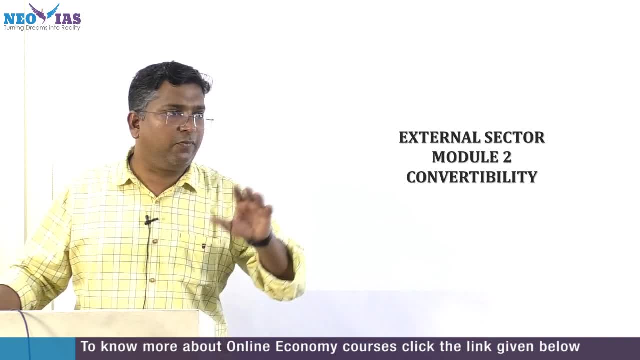 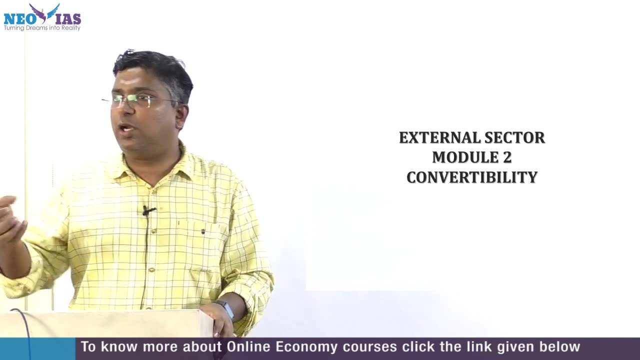 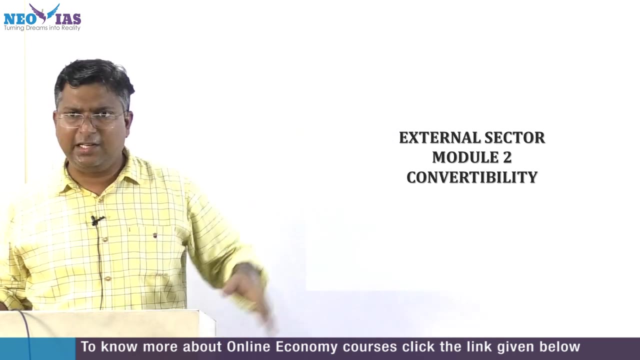 Their features of an hard currency is that they are not volatile. Their values almost stable throughout a certain period, their values stable and they are highly liquid. highly liquid means that dollar, if you have dollar, you can easily convert into Indian rupee. you have to just go to this marine drive or that. there are certain even 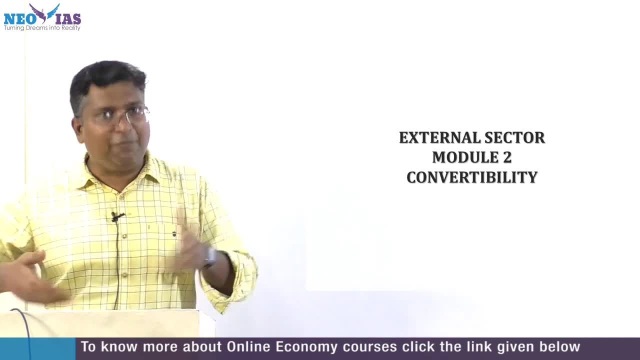 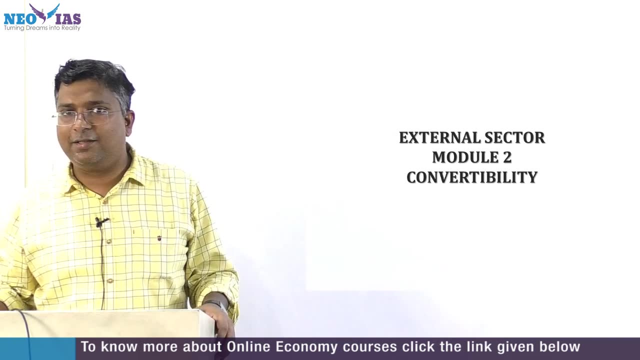 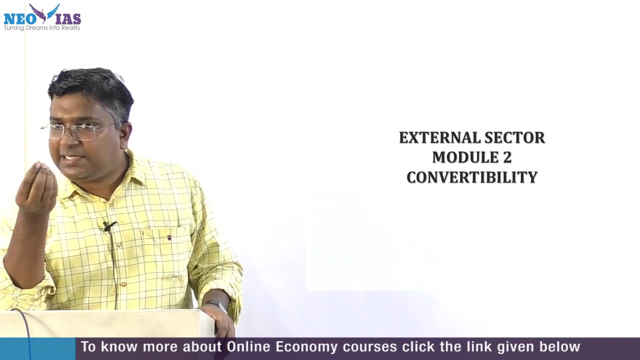 there are two categories: officially, you can convert. unofficially also, you can convert if you go to that place, Broadway. if you, if you are a foreigner, then, sir, you want dollar, they'll come to you. so what? what is the difference is that you have to pay only less Commission, but if you go through these money transfer. 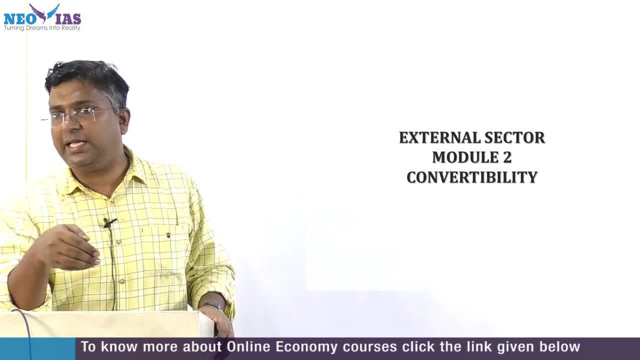 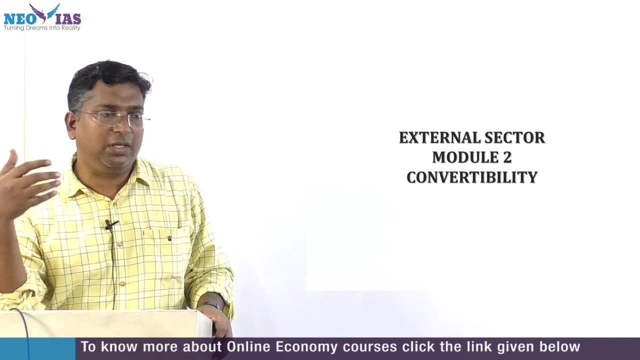 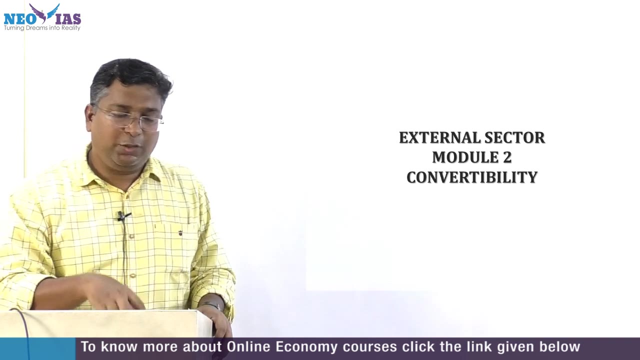 channels, and now there are many there. they will charge you extra so you will prefer that. but one is legal, other is illegal. but we are not, unless and until that money is not used for me negative purposes, like terror or other theater activity or other, and in Excel activity. otherwise, to an extent it is not a. 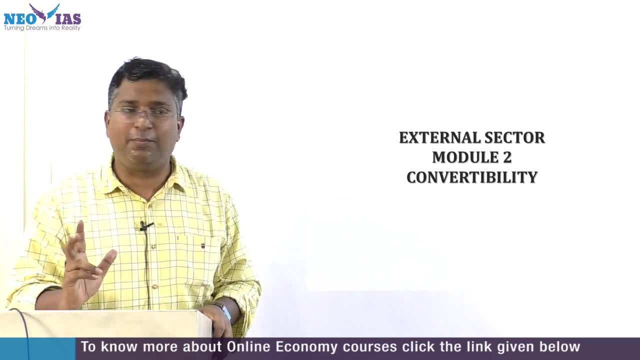 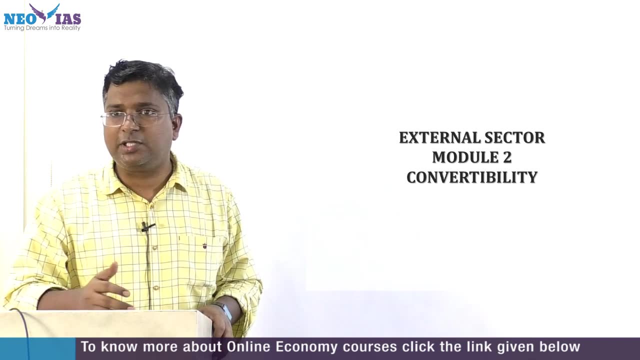 problem, But everything starts in a small manner and reaches a big amount. okay. Or gold smuggling: everything happens there like that. only See, Kerala is famous for gold smuggling. you know that? no, Yes, See, you are hearing news in the customs. 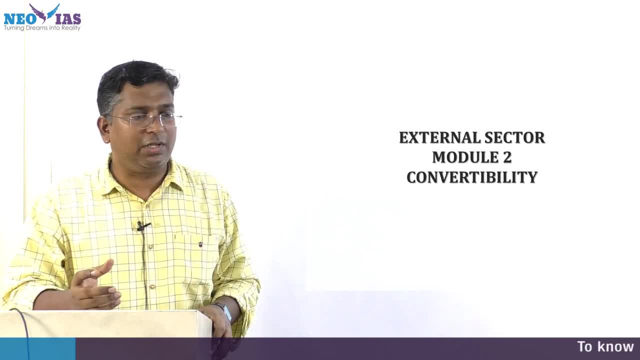 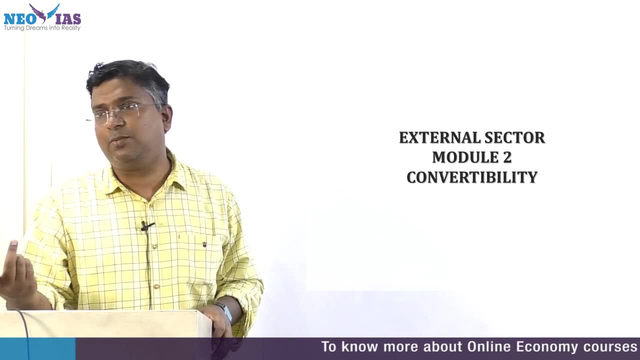 Actually, if 1 lakh- I am just giving an example- okay, If 1 ton of gold reaches here only, maybe you can say 1 kg, they show, Otherwise they have to show something, Something. they are this thing, okay. 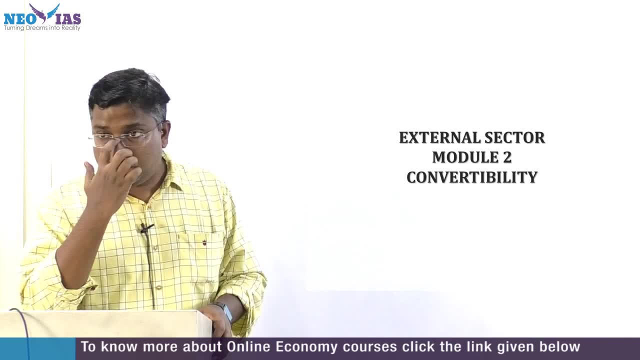 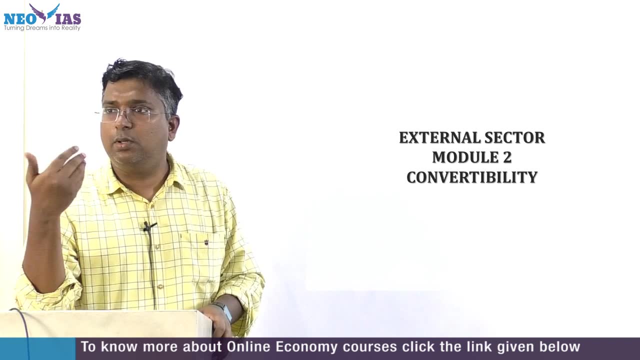 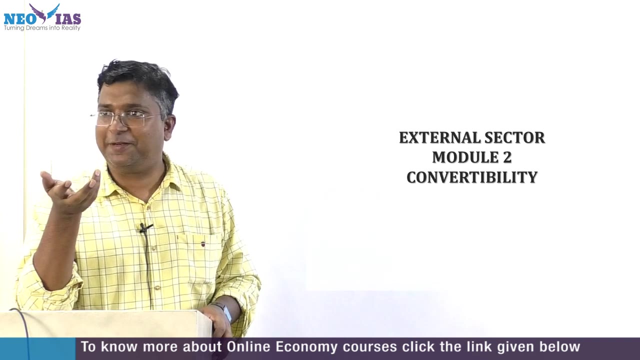 So all are. actually, they are not legally reported and they are not reflected in the balance of payment also. Okay So, but as the time grows, okay now it is very difficult for these smugglers to do business in India, Not only in India, everywhere. 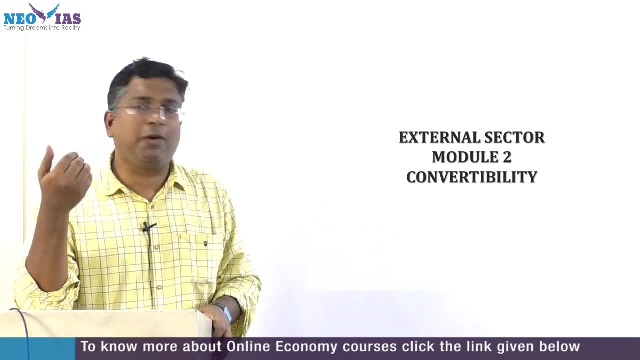 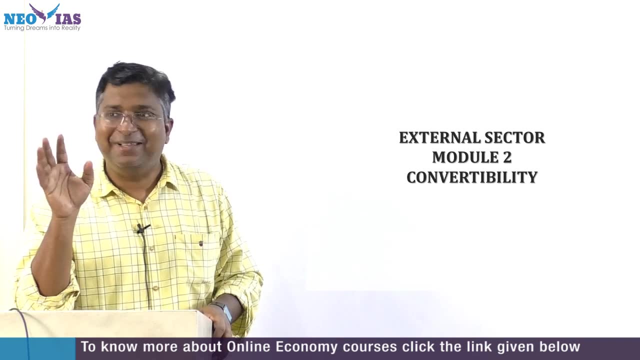 Because one way or another, in one chain they will get caught, because all our movement is there. If you are carrying mobile means wherever you go, I will be there Means- the US GPS will be looking at you. okay, You are doing this. 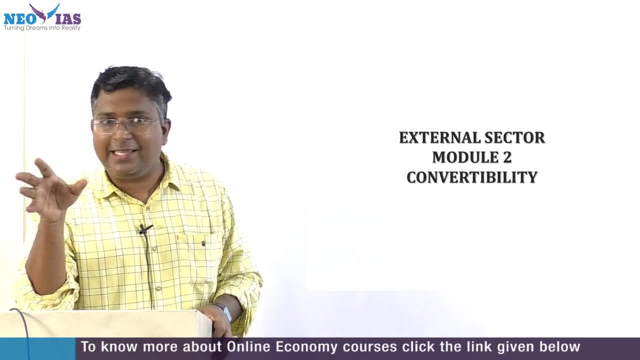 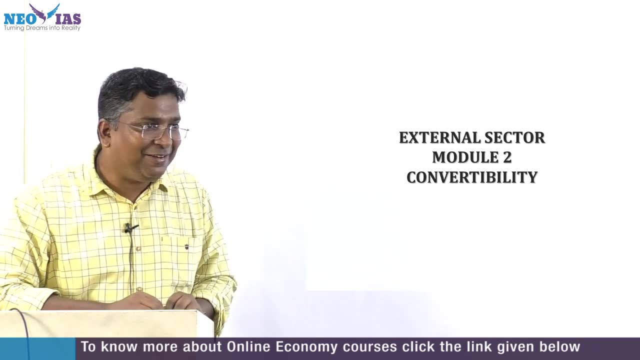 Now they will know that this number of 5, 10 students and a teacher is taking classes From US White House. they will be seeing it. Similarly, we have a small White House in Delhi- PMO. They will also be watching, okay. 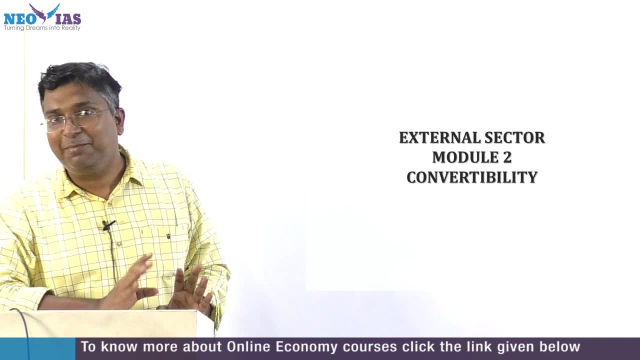 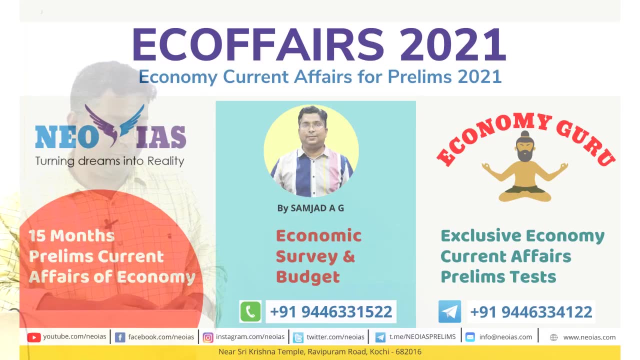 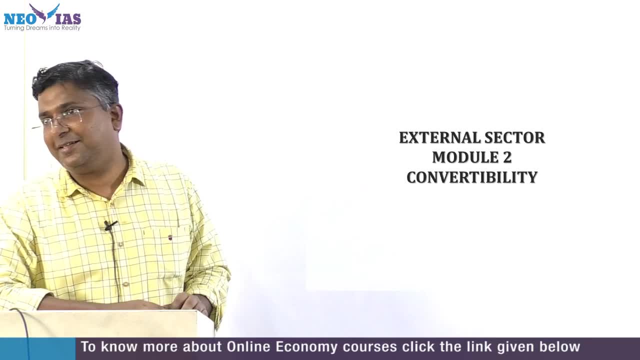 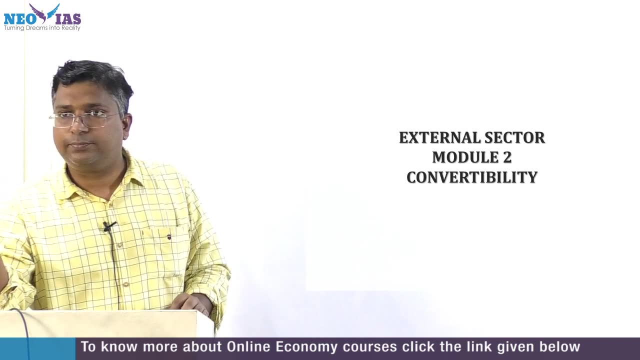 very difficult for IS IPS officers because they are waiting, okay. Anyway, what I am trying to say is that illegal things is not reflected when it comes to Havala transactions. They are not Havala, you know we will convert. So all are a pity that there is a system. they have a better system than our own government system. 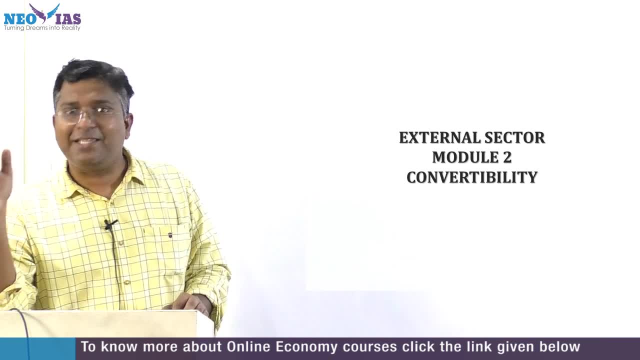 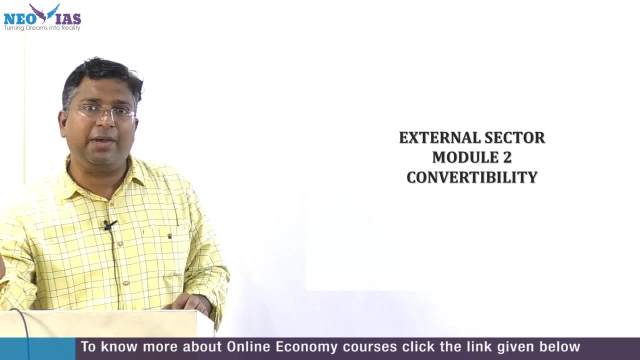 They are more secure, they are more confidential, they are more sincere. okay, So that is it. That is the reason why they have been so successful. They have a chain of command. If one person gets caught, they will. who is the real person? they cannot? it is all these things you have seen in movie. okay, 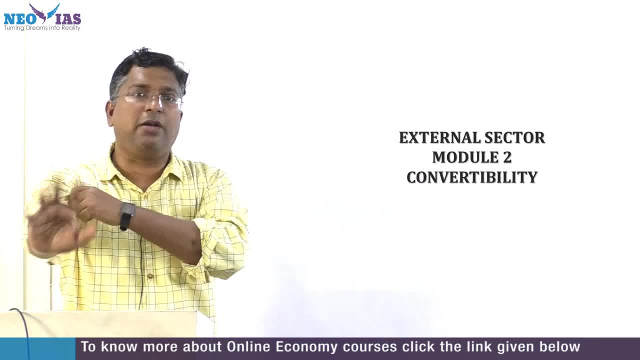 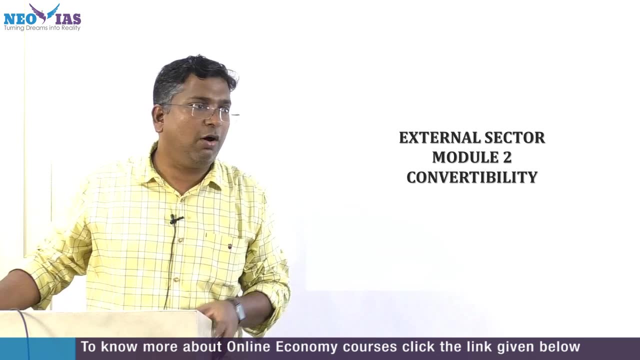 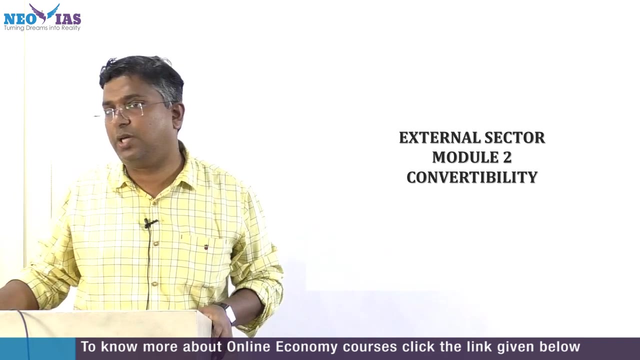 Anyway. so, regarding convertibility- because convertibility is all about that- okay, converting one currency into another. Now, why we reserve these hard currencies like US dollar, is that because of its stability and liquidity. You know the meaning: stable means the value will be stable. liquidity means you can easily convert into cash. okay, 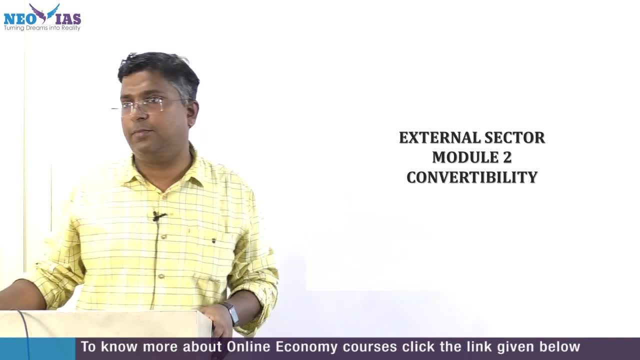 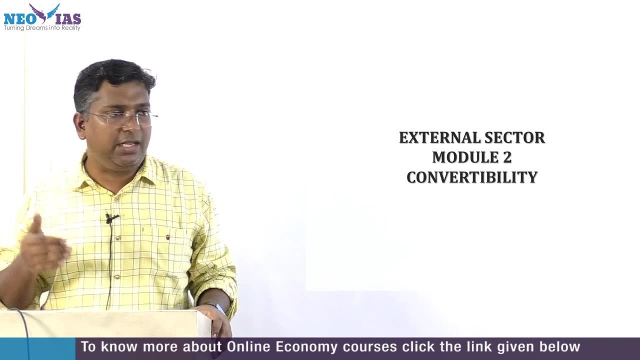 So convertibility is nothing but your freedom. It is a right. convertibility is a right of an resident individual who is staying in India. A resident individual who is staying in India, he or she has the right to convert the domestic currency- in India's case Indian currency- into foreign currency, and vice versa. 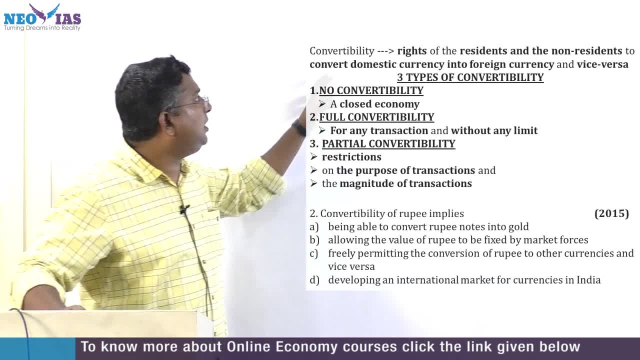 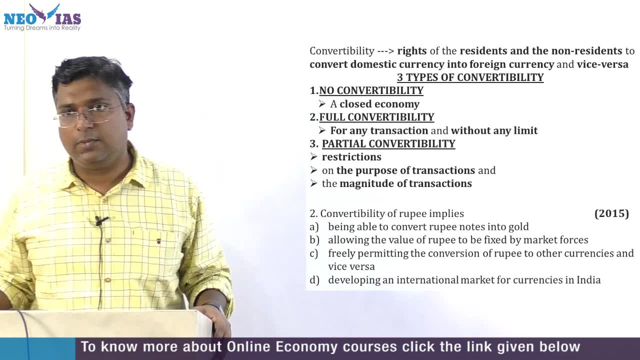 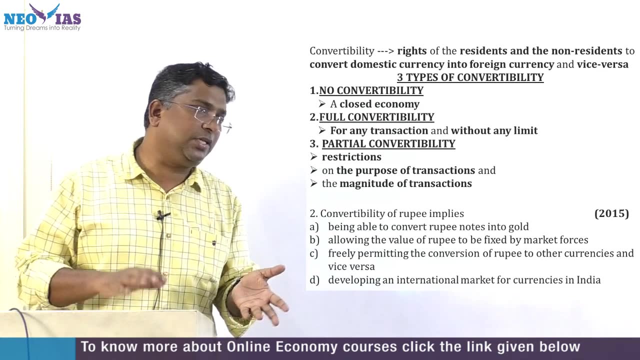 That is what is called as convertibility. So convertibility is nothing but the right or freedom of a resident as well as non-resident, you know, to convert domestic currency into foreign currency And vice versa, foreign currency into domestic currency, domestic currency into foreign currency. 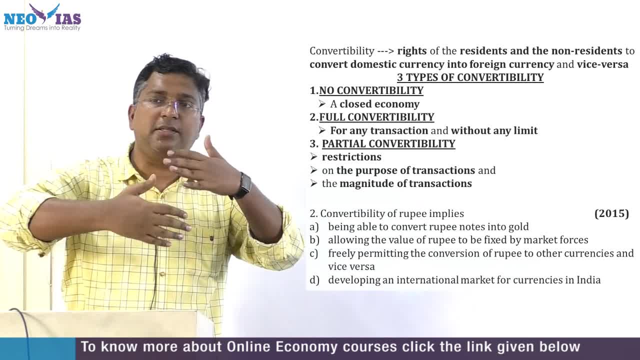 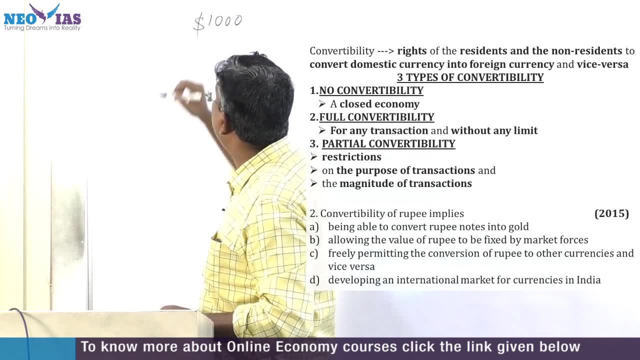 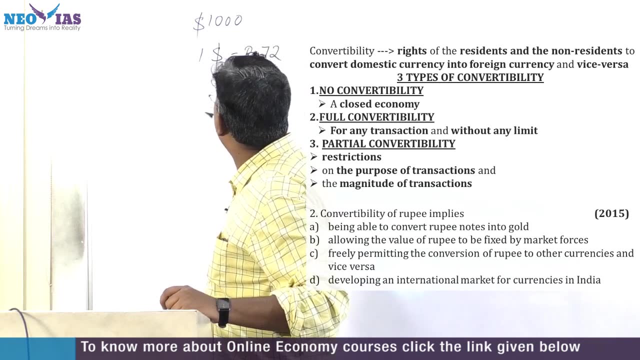 So conversion, so convertibility, is nothing but converting one currency into another currency. For example, if you have thousand dollar, you are having thousand dollar. okay, and one dollar is rupees 72.. So what you can do, you can see. I am not talking about commission charges. 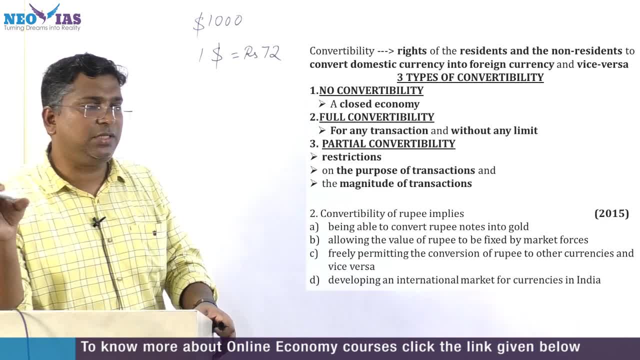 There will be a commission charges will be there, But we will talk about commission charges later. But we will talk about commission charges later. So without taking into consideration commission charges, so you can convert thousand dollar into seventy-two thousand rupees. 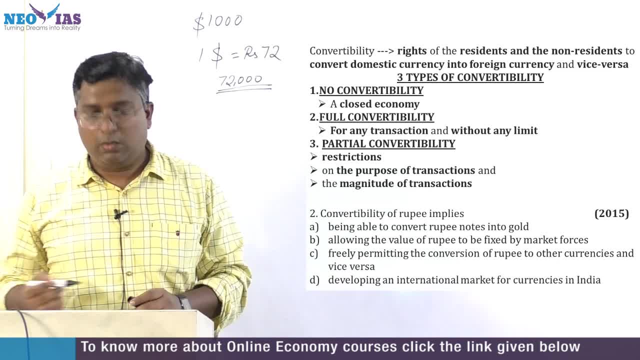 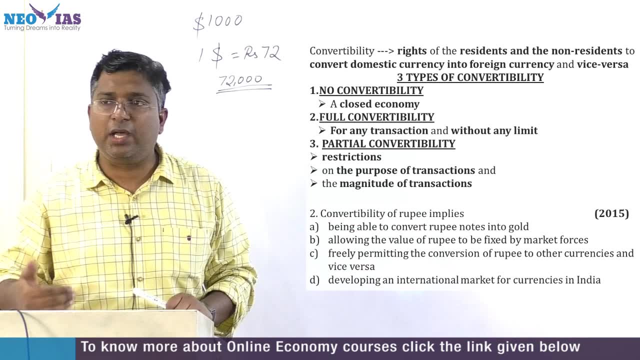 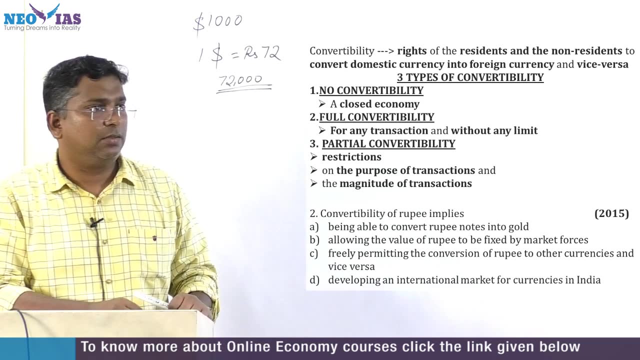 This is convertibility. Now, this is one way of domestic currency converting into sorry foreign currency, converting into domestic currency. Similarly, if you are having seventy-three thousand, you can convert into thousand dollar by considering the commission charges. So two different way: domestic currency into foreign currency, foreign currency into non-domestic currency. 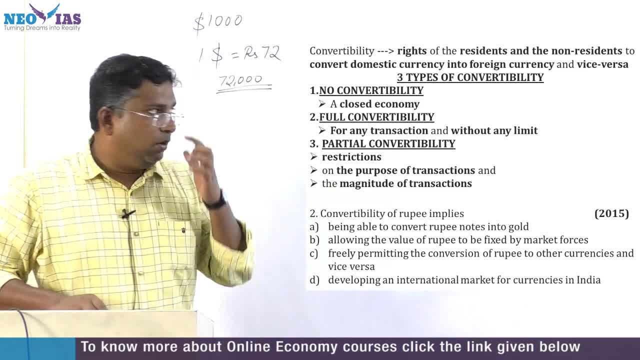 So two different way: domestic currency into foreign currency, foreign currency into non-domestic currency. That is the meaning of vice versa. Okay, so we know. so are you clear with convertibility. They asked a very simple question: what is convertibility? 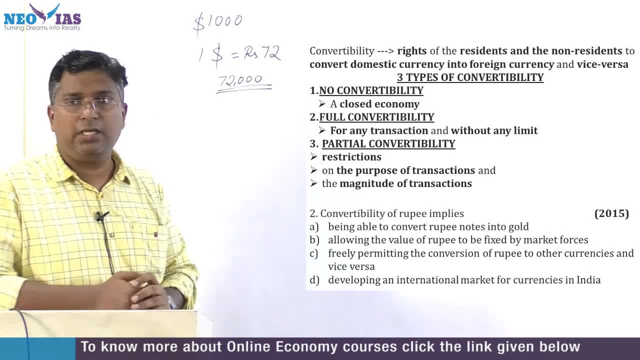 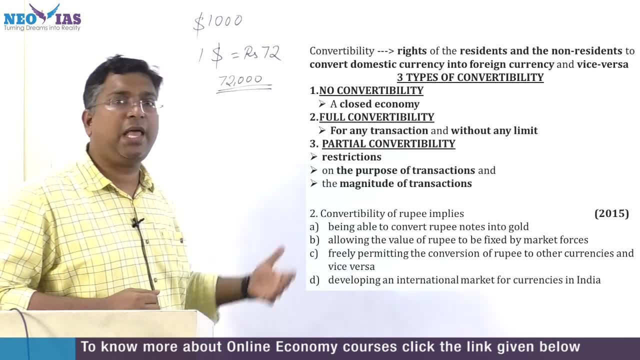 Okay, see the 2015 question In the year 2015,. they asked a question. simple question: Convertibility of rupee. they are asking about convertibility of rupee Implies. what does it imply? Being able to convert rupee notes into gold? is it correct? No, Allowing the value of rupee to be fixed by market forces. No, So freely permitting. freely permitting the conversion of rupee to other currencies and vice versa. See is your answer. A simple question. 2000 year is 2015.. 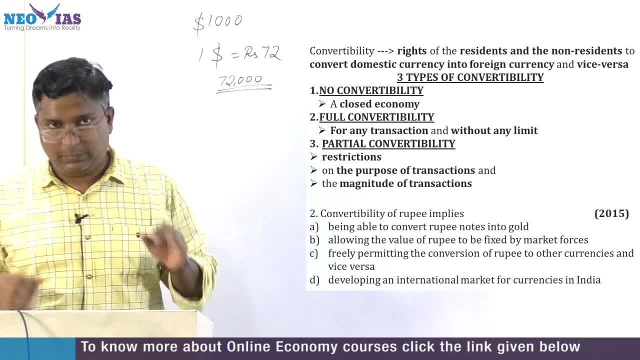 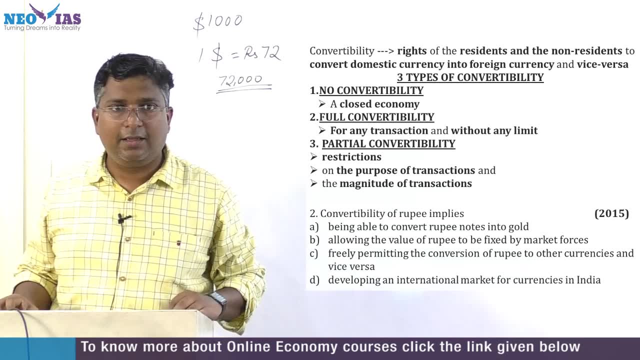 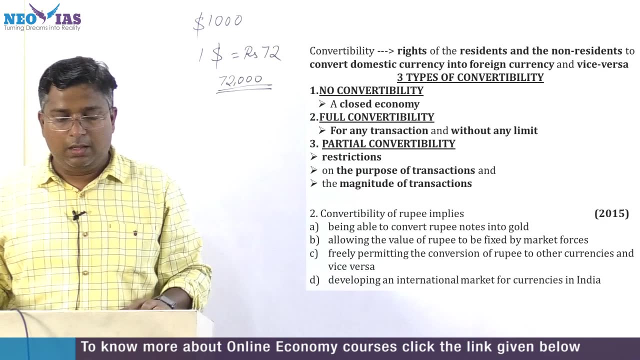 Now there are three types of convertibility. There are three. where is Anaga? She is missing. Yesterday also she was not there. Okay, Okay, no convertibility. See from the term itself. see every country follow any of these convertibility regime. 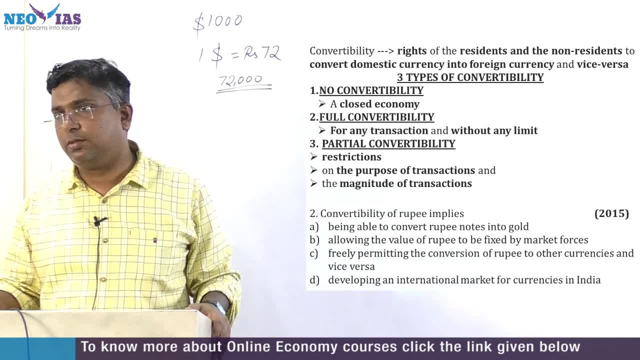 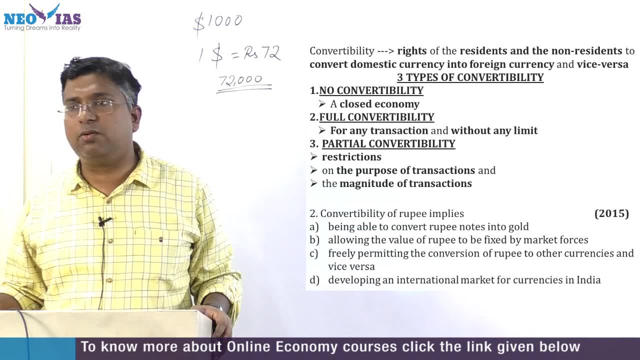 Either they will say that they don't, they don't allow conversion, That is, that country follow no convertibility regime. Some countries will allow full convertibility- I will explain what is full convertibility and no convertibility- And some allows partial convertibility. 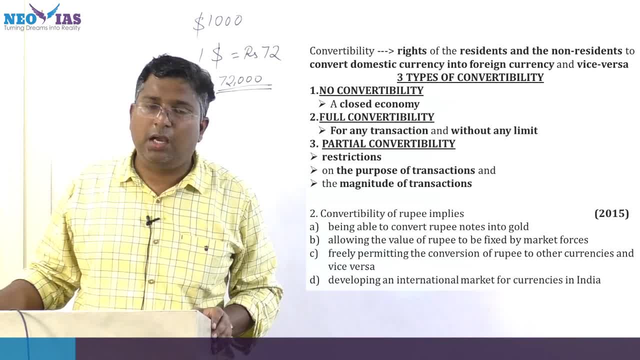 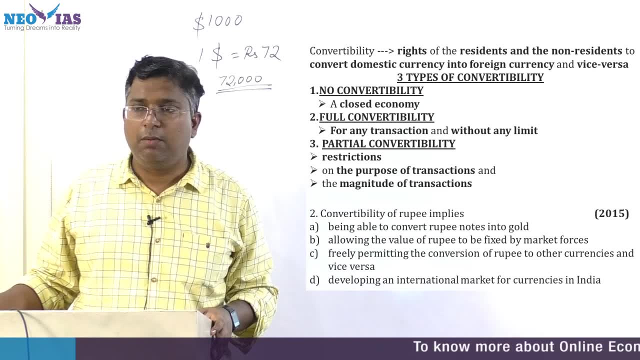 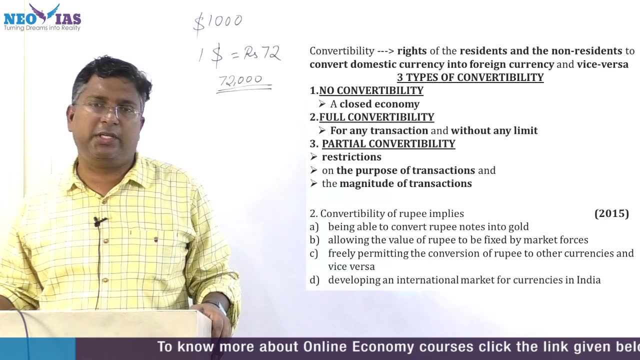 In India we are having partial convertibility. India is having Countries like US, Canada, European Union, even Russia. They are having full convertibility, Okay, But majority of the countries are having partial convertibility. Ideally, there is no country which is having no convertibility. 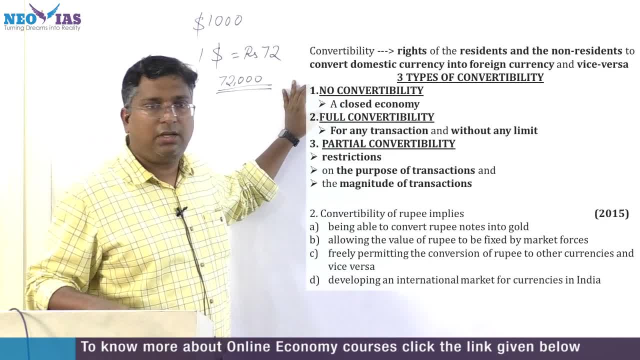 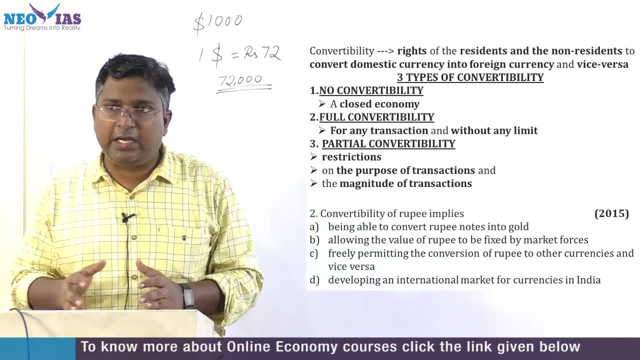 So this is now only an idealistic situation. Either countries will be full, having full convertibility or partial convertibility. So now I will, in order to understand no convertibility for a country to become no convertibility regime, which India tried after 1947.. 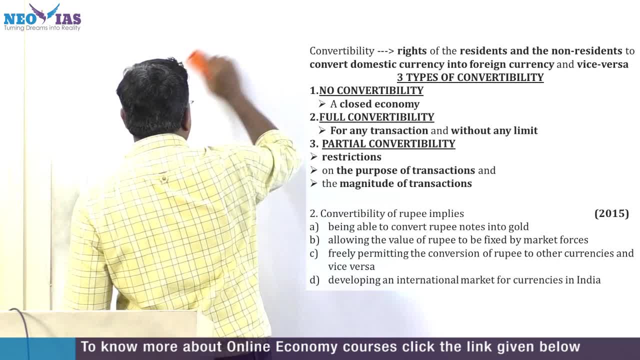 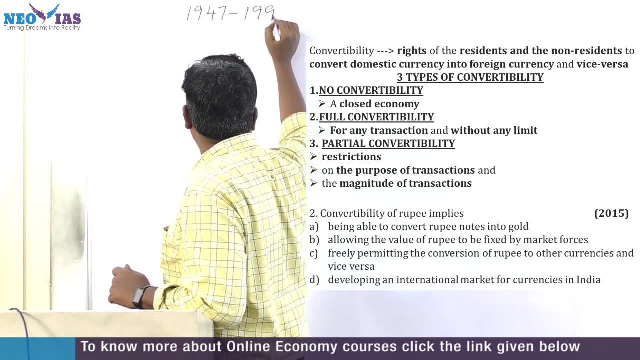 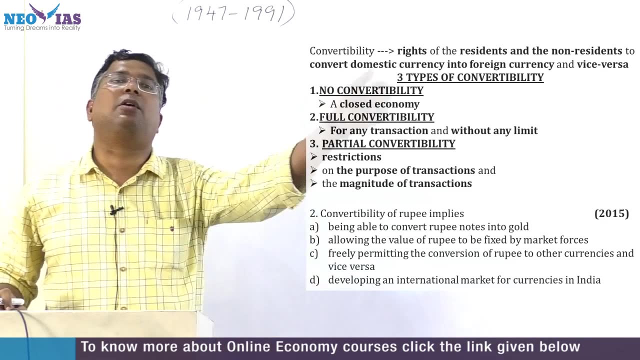 Okay, India during this period 1947. 1947. To 1991, was a closed economy. only in a closed economy, no convert, no convertibility is possible. In this time period, after independence till economic reforms was launched, India was almost a closed economy. 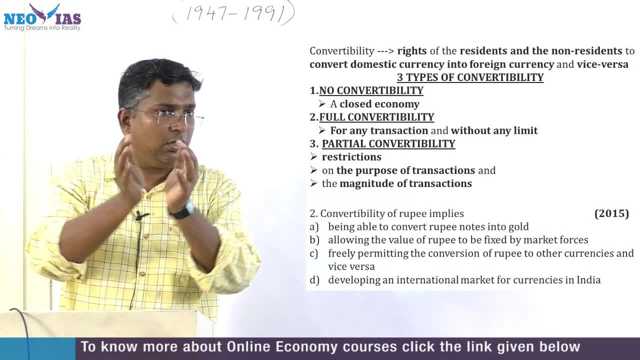 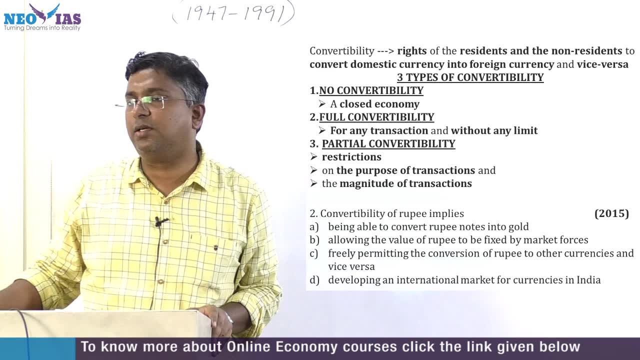 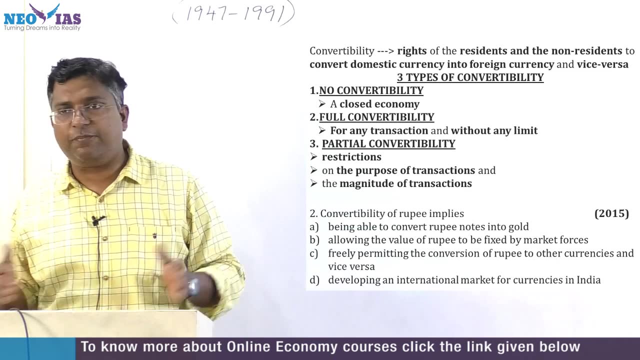 Closed economy means we never allow import. complete economies closed only. transaction will be within the domestic transaction. domestic trade, no international trade, no international transaction. Okay, So no international transaction, etc. No imports, no exports, no capital movements, no FDI, no FPI, no external loans, etc. 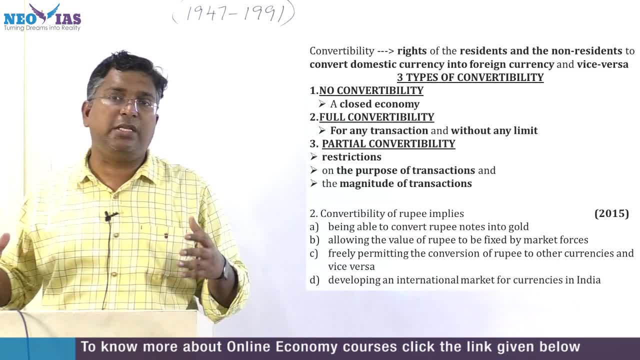 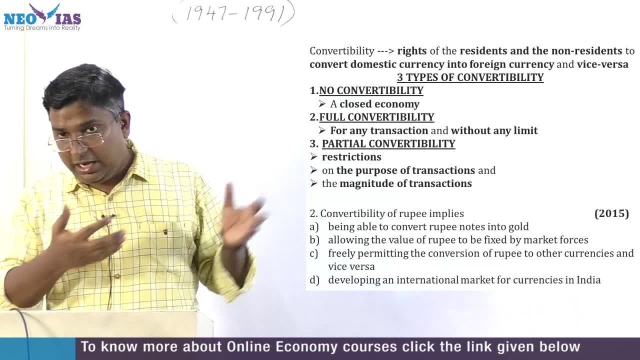 But even though we were a closed economy, unfortunately, due to the India's peculiar situation, In 1940s, late 40s and 1950s and early 1960s, we were importing food grains due to severe droughts. 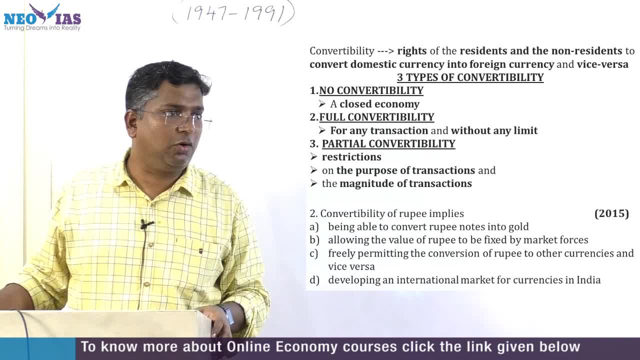 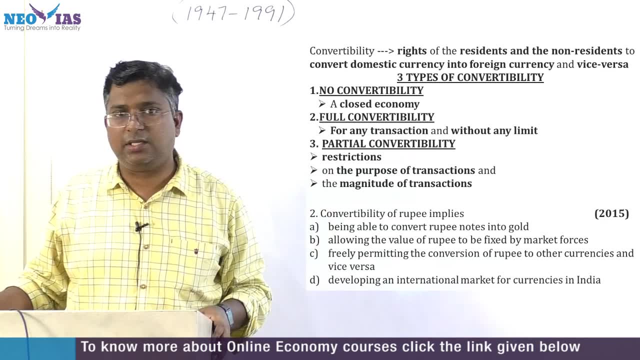 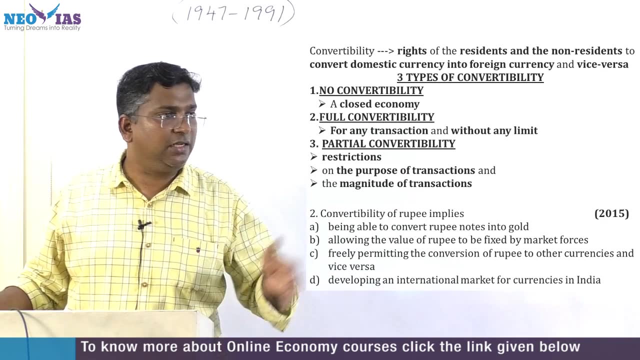 But after we implemented green revolution that problem was sorted out. But we, as part of the second five year plan, As part of industrialization, we started importing heavy machineries, capital goods. So one way or another then we started after 90s, 1970s, we started importing petroleum products. 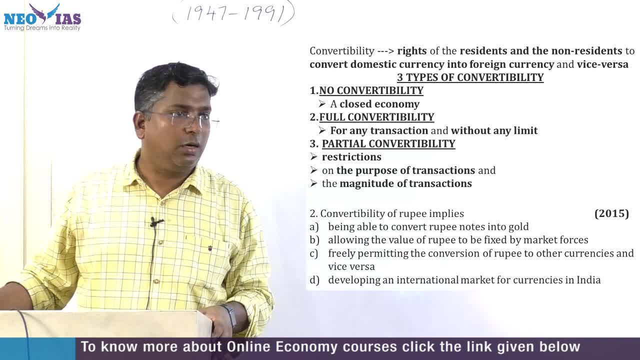 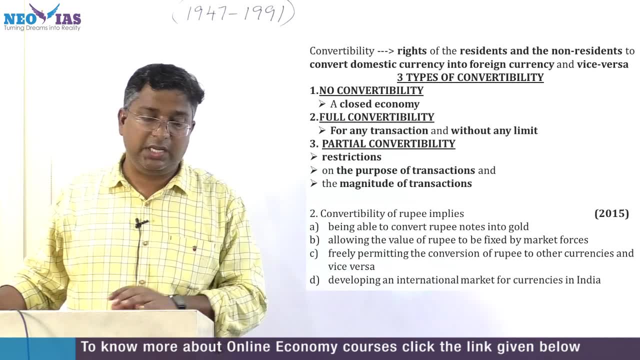 All makes India. even though India says to be a closed economy, we were not a closed economy. Okay, So that we will discuss in detail regarding closed economy in detail in foreign trade policy module. Okay, So are you clear. with no convertibility. 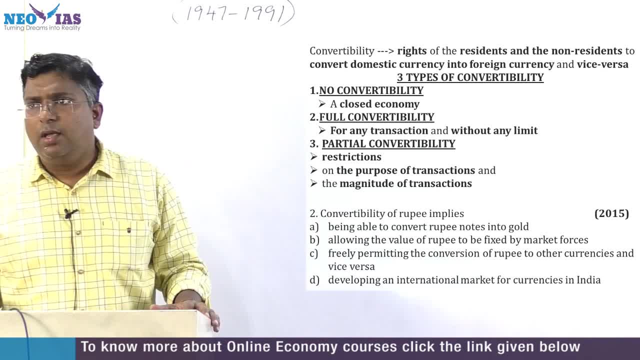 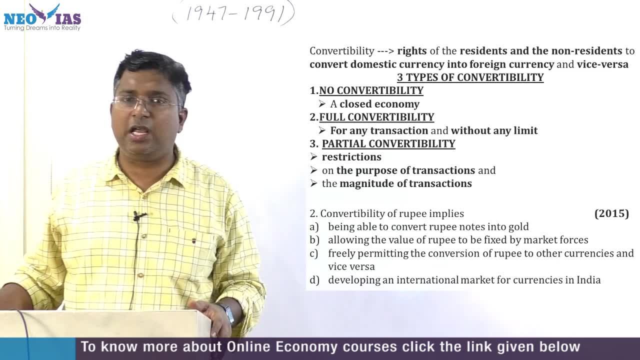 Okay, Now full convertibility. See, now try to understand. full convertibility means like: suppose you are a crorepati. Imagine you are having, you are a crorepati in India. You are having a massive wealth of 1000 crore. 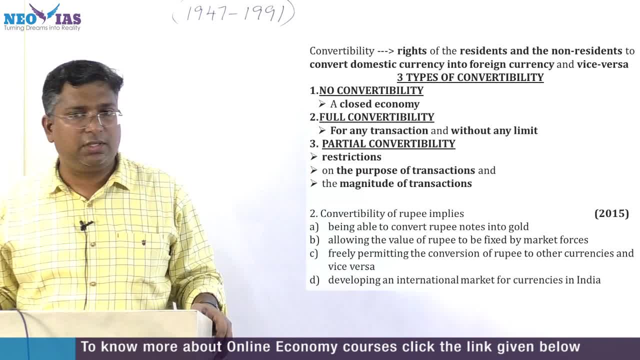 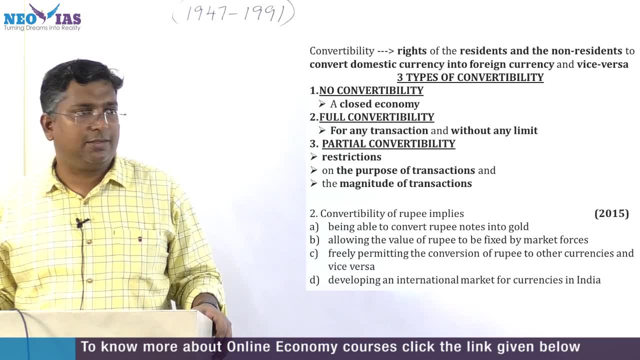 And in that, 200 crore is in cash in different bank deposits like that, FDI, etc. Now you want to purchase a palace in Buckingham or in UK, whatever it is, If you, if they are ready to sell. 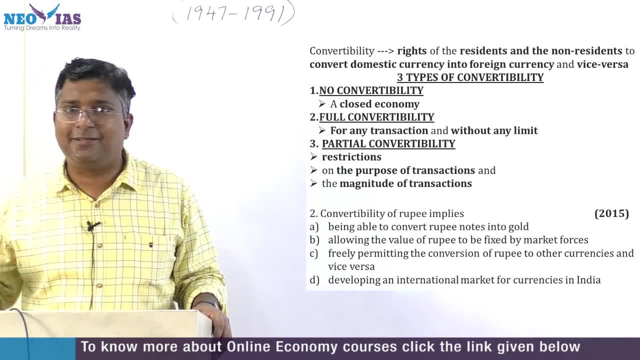 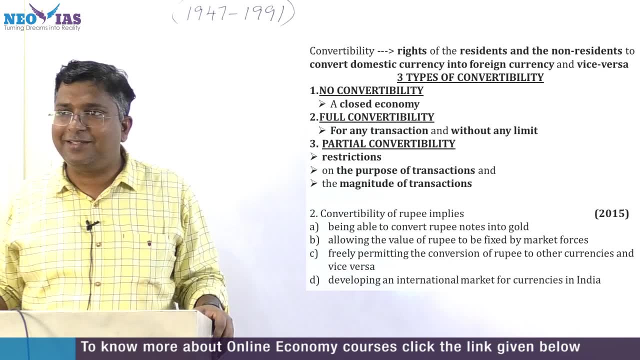 You can buy in IPM money. Or if you want to buy an island, you know when the film stars have their own islands, Okay, So they can all buy it. But in that case the Indian government will say that where are you going? 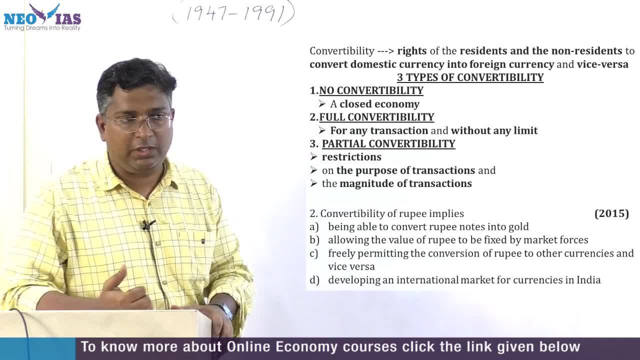 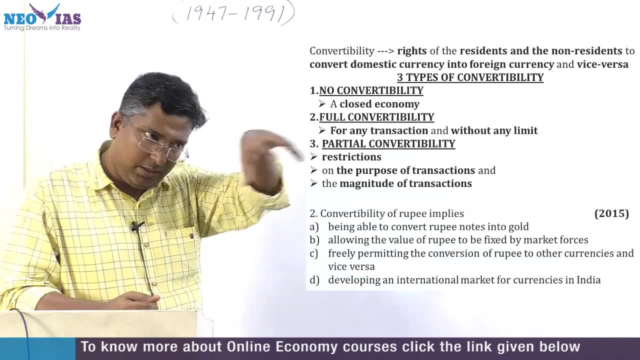 See if you are now. what is the problem is with this convertibility, full convertibility. Okay, So they have to convert Indian rupee into foreign currency? Where? In India, in the Indian continent itself, In the, in the Indian foreign exchange market. 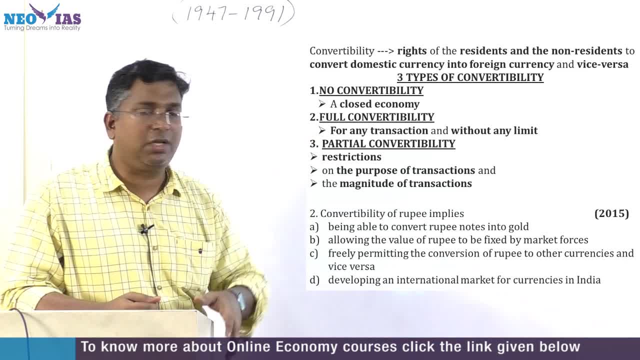 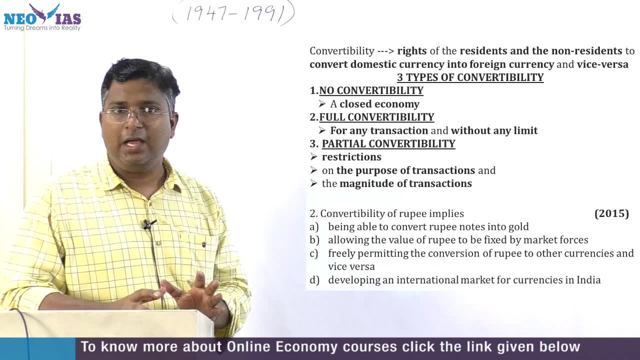 So there is a market for foreign See, where, Where conversion happens in a market, what is called as foreign exchange market. Everything is now integrated online, But everything happens in India. We have a foreign exchange market. What is the function of a foreign exchange market? 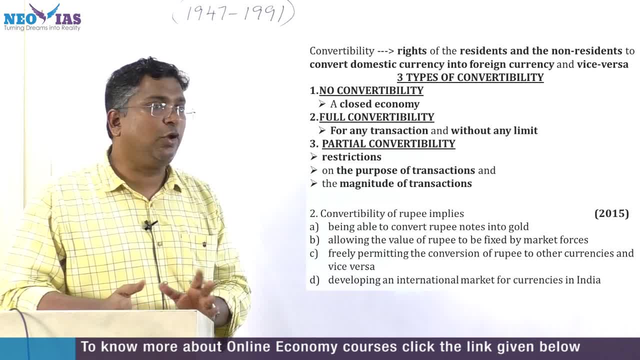 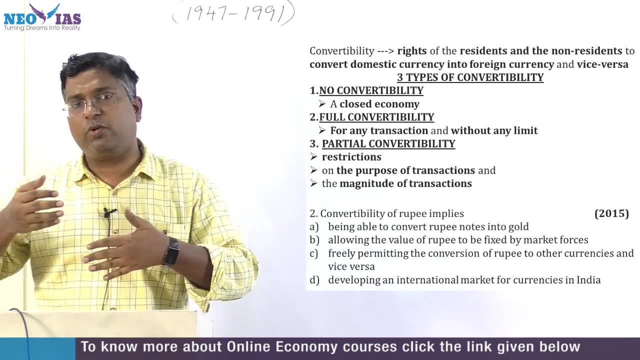 Here foreign exchange. Foreign exchange is nothing but foreign currencies. Foreign currencies are traded, So there is daily sales. daily sale is going on, Converting Indian rupee into dollar, dollar into euro. like that it is happening in the foreign exchange market. 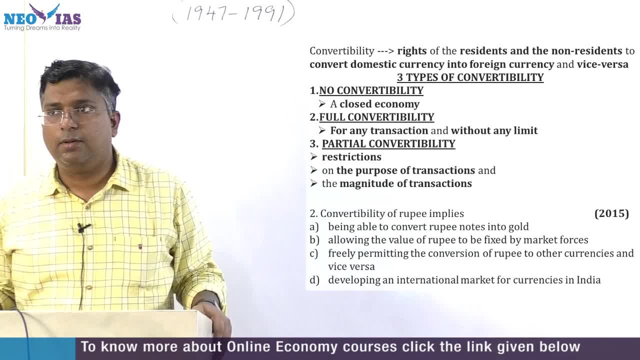 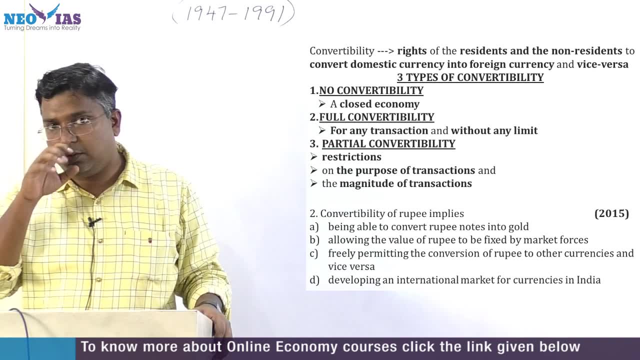 In foreign exchange market, only currencies will be traded. Okay, we will come across different terms, what is called as currency war currency. we will come to it, okay, slowly, we will come to it, Okay, So are you clear. what is foreign exchange market? 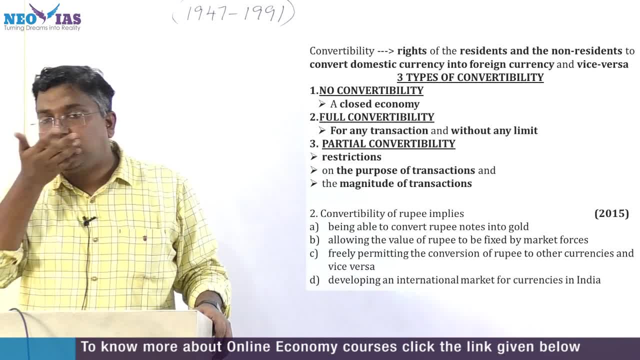 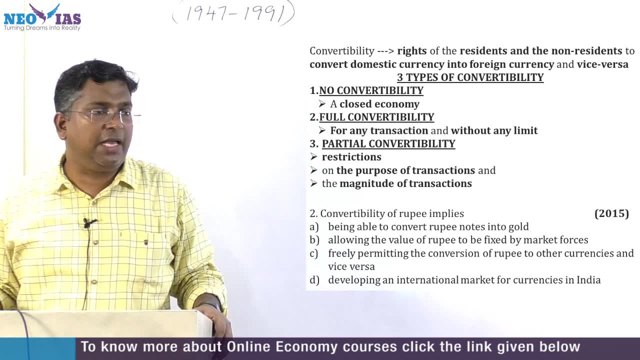 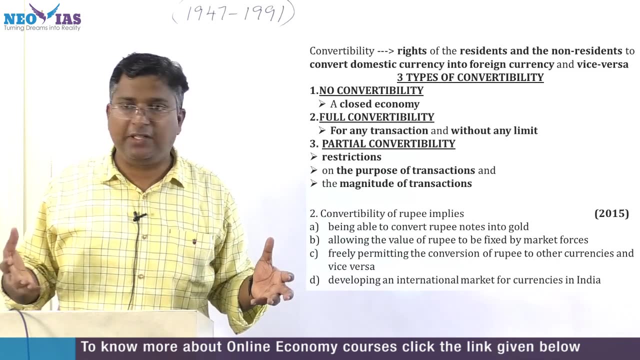 It is a market where foreign currencies are traded, So there are genuine, there are regular people like importers and exporters who will come to convert their currency. For example, exporter will come to foreign exchange market because exporters have got, they made a shipment and they received $75,000. 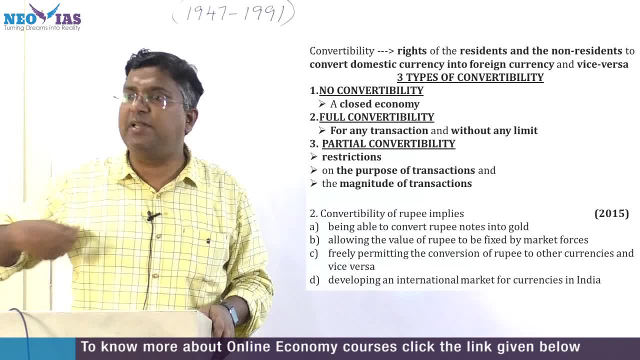 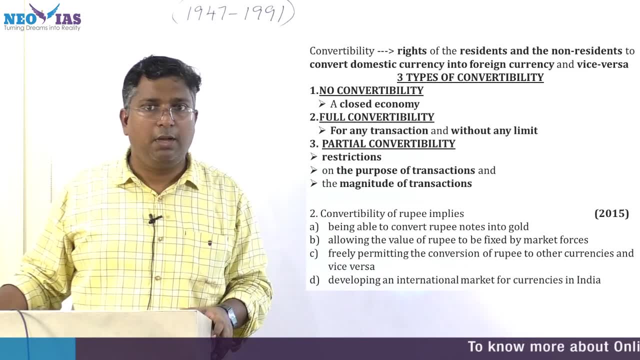 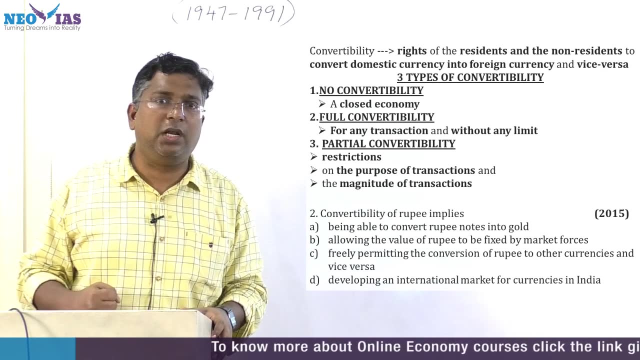 So what the exporters will do, What the exporters will do in the foreign exchange market: they will sell the dollar and take Indian rupee and then they will settle all their dues. But, importer, they are having Indian rupee, they want to import. they will go to the foreign exchange market and get dollars and then this dollar is paid to the imported company. importing company. 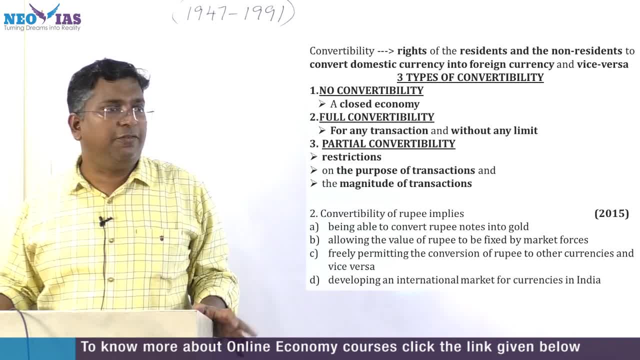 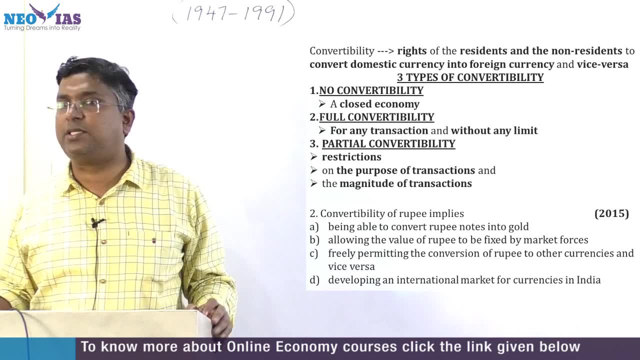 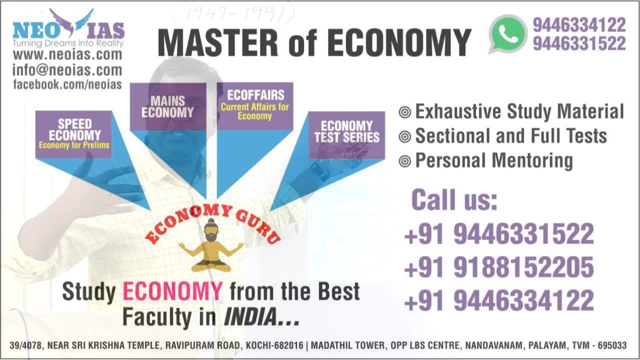 Like this is happening in the foreign exchange market. okay, So here, so in full convertibility regime. India is not a full convertibility regime. Okay, Like US or European Union, you can. there you have the freedom to convert any their domestic currency without any limit. 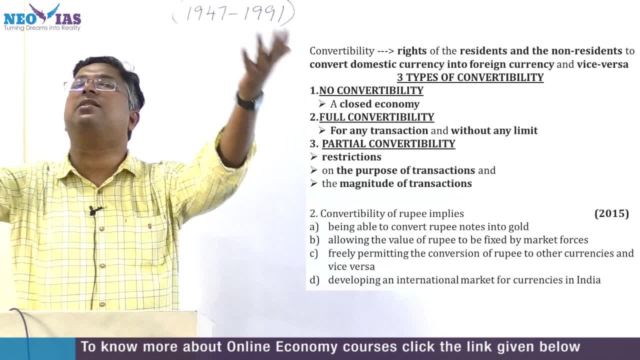 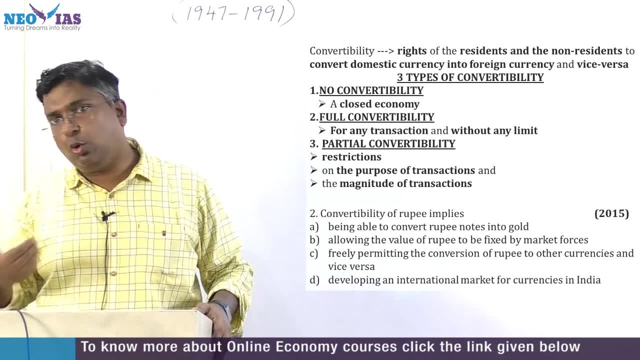 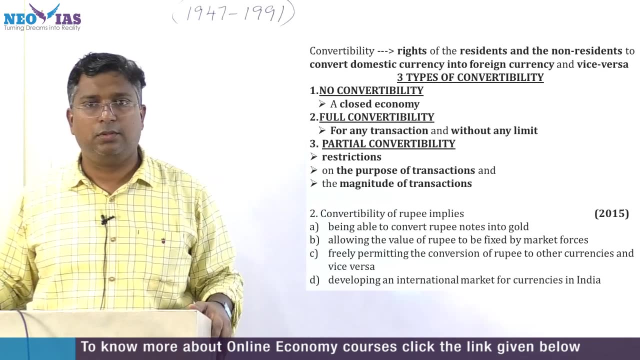 There is no limit. You can conduct as much as for any transaction. the government will not. you can. you can do any transaction: import transaction, export transaction. You can borrow through external commercial borrowing. Okay, So any transaction for any transaction and there is no limit. also, 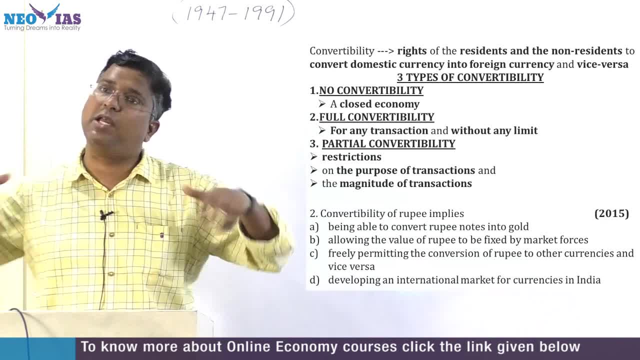 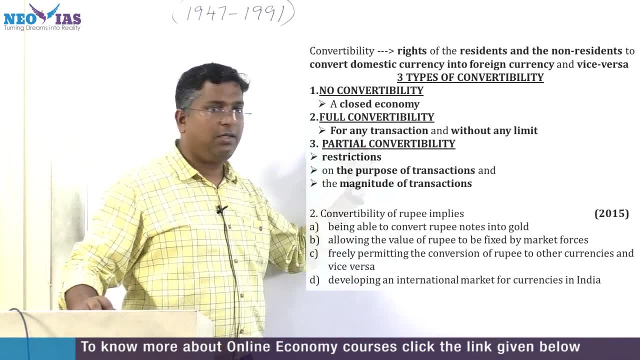 You can bring 5 crore, 10 crore, 1000 crore, or you can invest 1000 crore in foreign currency in a different country. everything is possible. So no limit is been set and there is no restriction on any transaction. also, 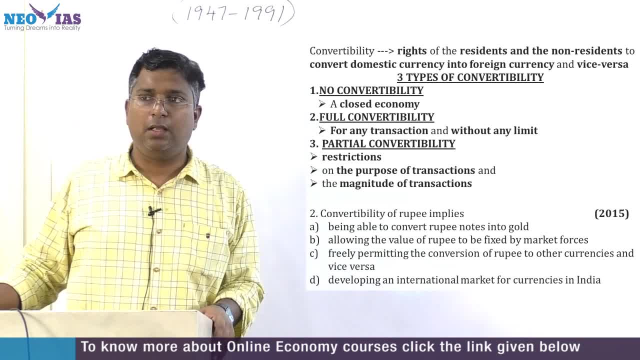 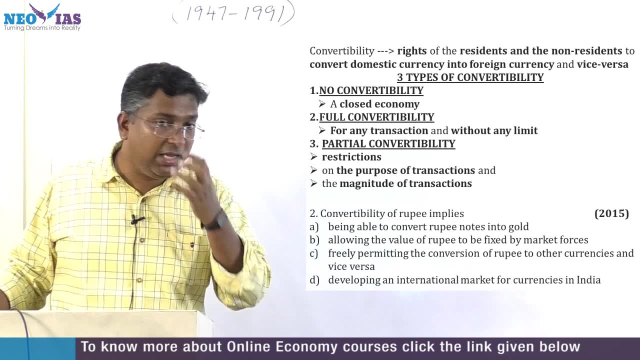 So that is what is called as full convertibility. But in India, if we do so, what will happen? is that why we did not went for full convertibility? Because already we are a country with current account deficit only, exception being 2021.. 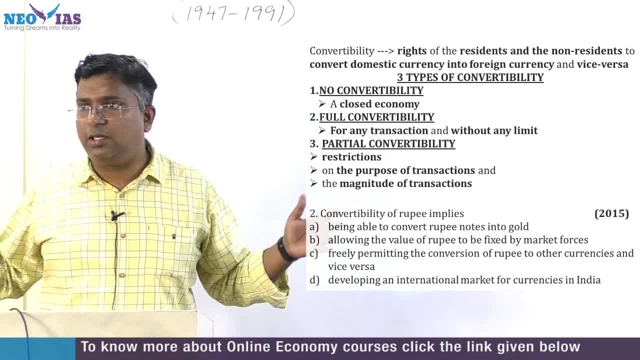 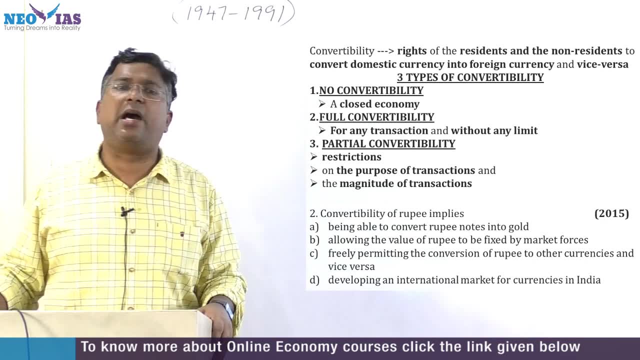 Because we have seen in module 1. In the last 40 years in the economic survey discussion I told you: Okay, Only once in a while we have current account surplus, But we are generally a current account deficit country. We are having BOP surplus because of capital account. 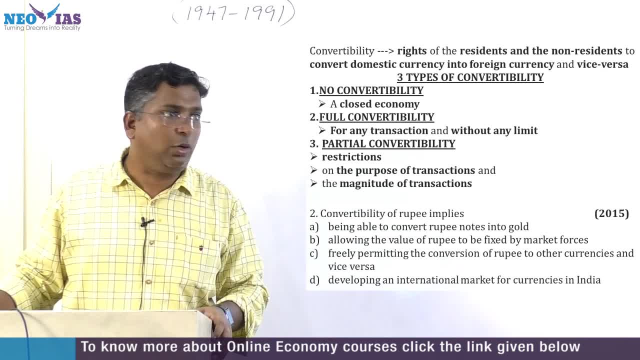 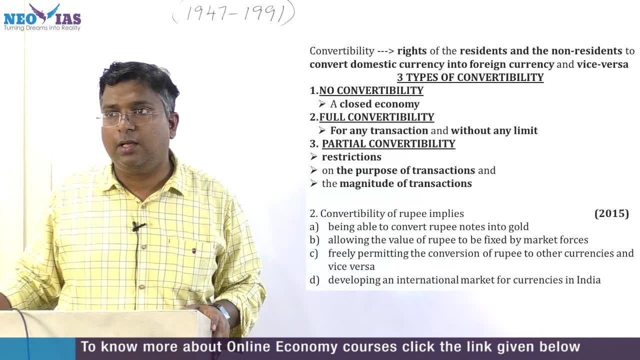 This capital, you know anytime it can go back to their own country. You cannot trust them. Current account surplus is the most safest thing. So already we are having current account deficit Okay, Plus when there is any global crisis. 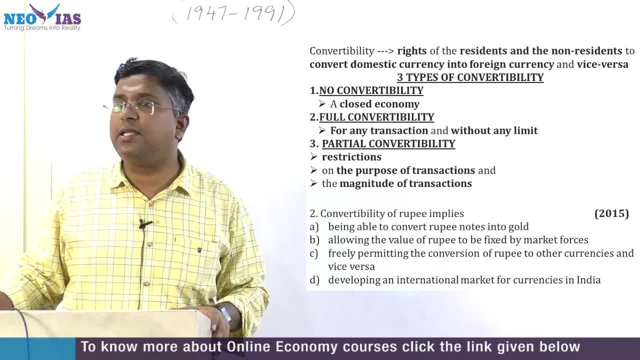 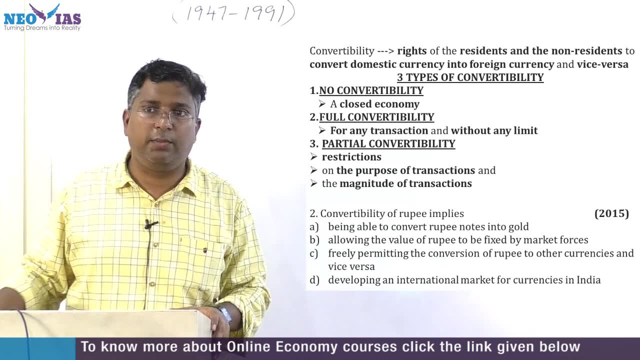 Okay, Global crisis, When there is any. this was the 2020 prelims question. Okay, At a moment. you know what this? there is a concept called as hot money. Hot money, Hot money. You know what is hot money? 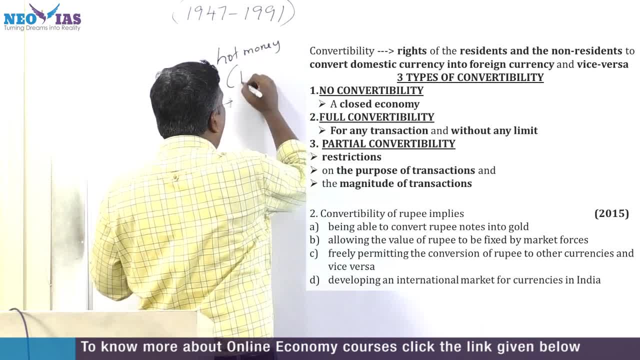 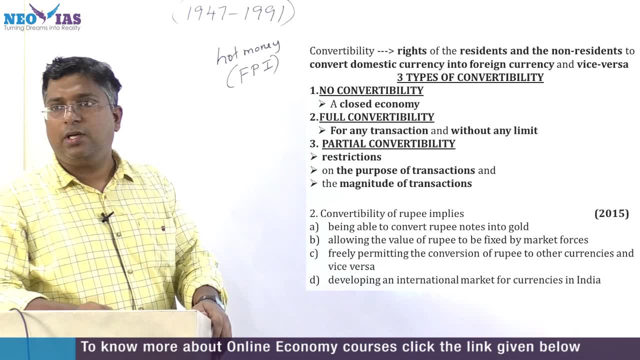 Hot money is nothing but FPI Foreign Portfolio Investment. When they hear a negative news- For example, in the election result will be coming on May 2nd- If they feel that it will create instability, The result will create instability in the country. Suddenly, market will crash. This market is crashed not by domestic investors, By foreign portfolio investors. They will withdraw the money and go to some other safe haven. So if there is any massive like global finance, What we are having If we continued- 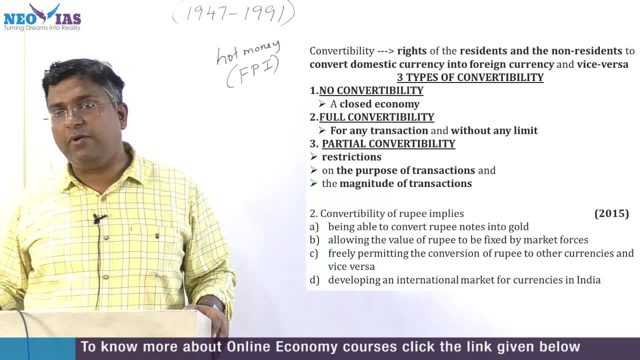 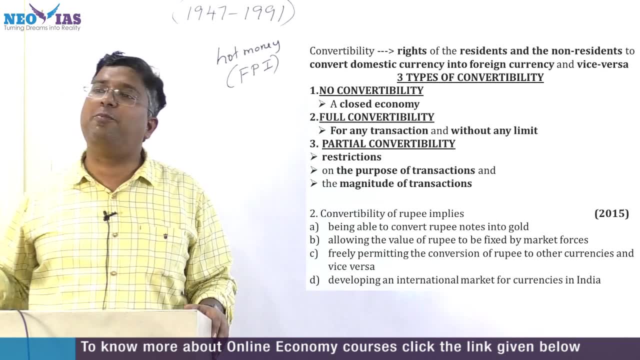 Now, very interesting thing, When we were under COVID-19 restrictions, Our stock market was rising Because foreign portfolio investors knows that, Okay, India is one of those country where in future there will be growth. Even the lockdown is for a temporary period. 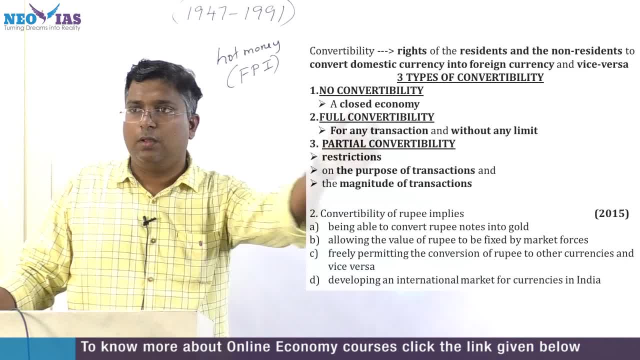 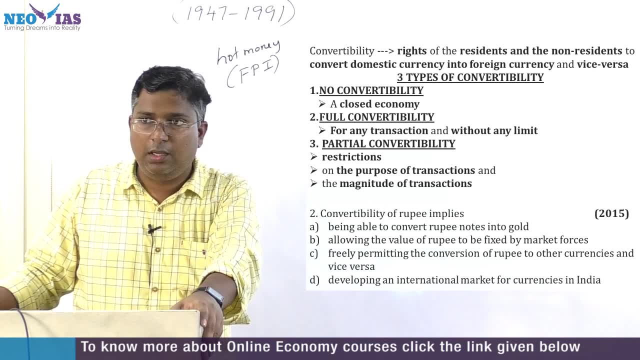 And they will come back. Okay, So that is So. if there is, If we, if we go for full convertibility, What will happen? Since we are having current account deficit And then we need a strong banking system? 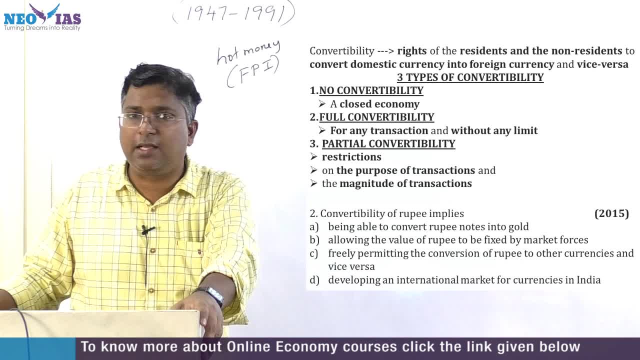 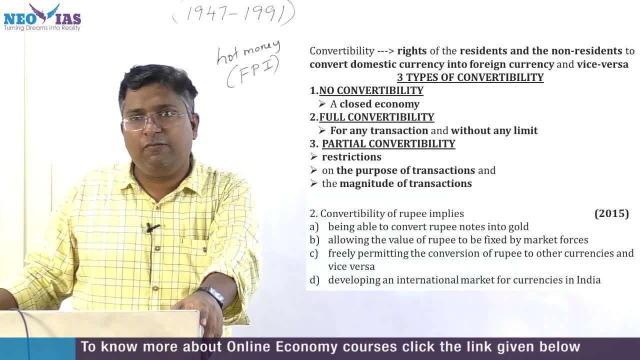 To implement it. We don't have a strong banking system. Many of our banks are losses, They are having huge bad loans And especially during lockdown it has worsened And we need to have forex reserve. But that forex reserve, We know that we have accumulated forex reserve. Mainly through capital account surplus only, Not due to current account surplus. So the condition is not ready. So anytime this foreign currency will go And it will affect the value of Indian rupee And it will affect the exporters and importers. 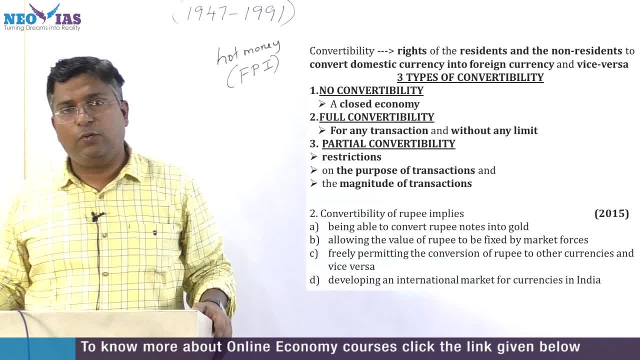 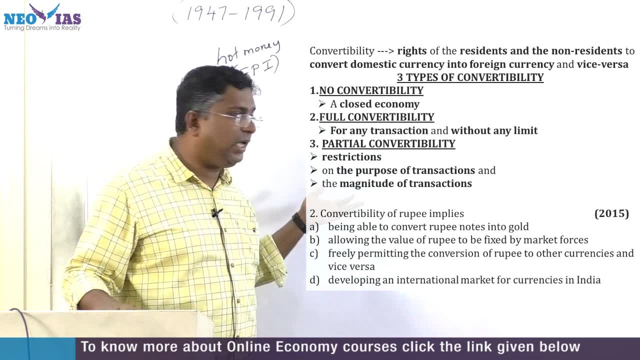 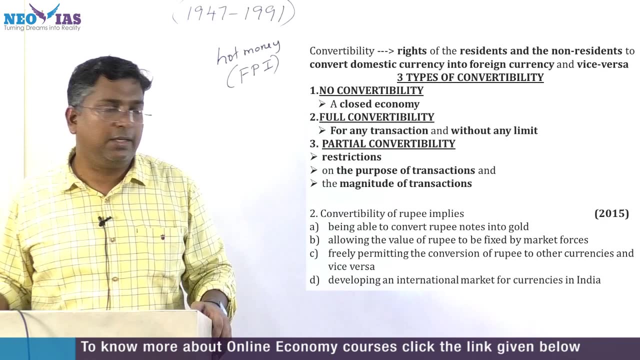 So we are not ready to implement full convertibility. Okay, So full convertibility is, without any restriction, You can, And without any limit Means you can convert the currency, You have the freedom to convert the currency. Now, partial convertibility is there are lot of restrictions.